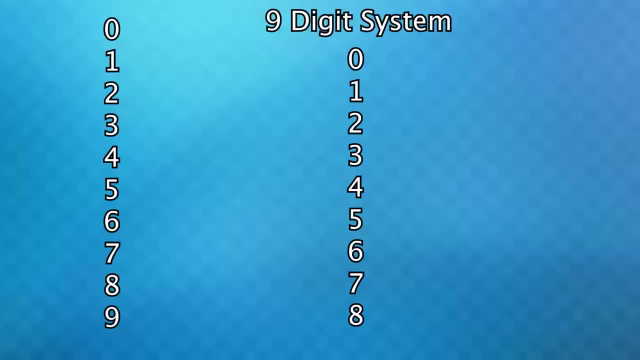 There's no reason we could not have 9 digits, which means after 8,, the next number would be 1, 0, because you'd be out of digits and you would need to reset the ones placed to 0, and then add a 1.. 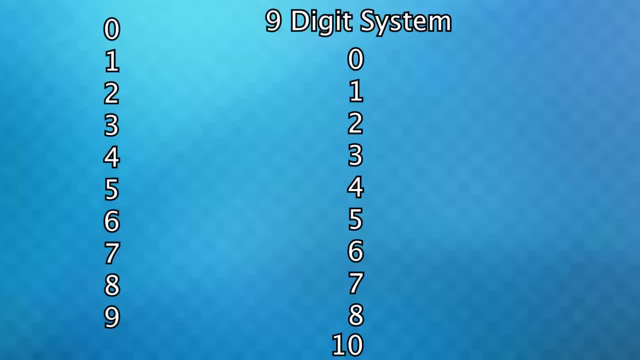 This would represent what we know of as 9,. if there were 9 digits, We believe that the 10 digits comes from the fact that we have 10 fingers. Simple as that. In fact, there are many times we only use 2 digits. It's known as binary. 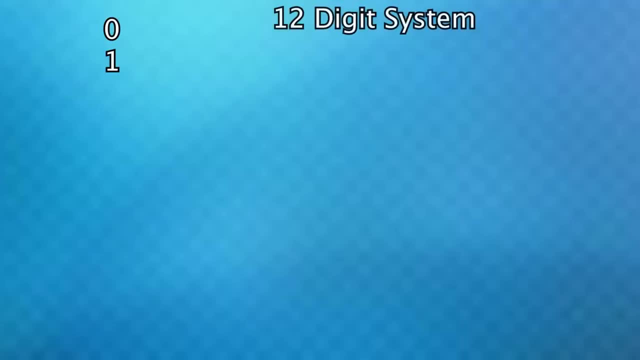 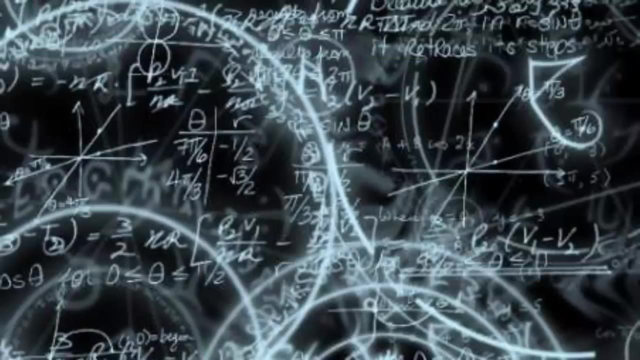 But mathematicians actually say: had we picked 12 digits, then arithmetic would be much easier, considering 12 is divisible by more numbers than 10.. Now, one of the oldest foundations of mathematics, which is lost on many people today, is logic. 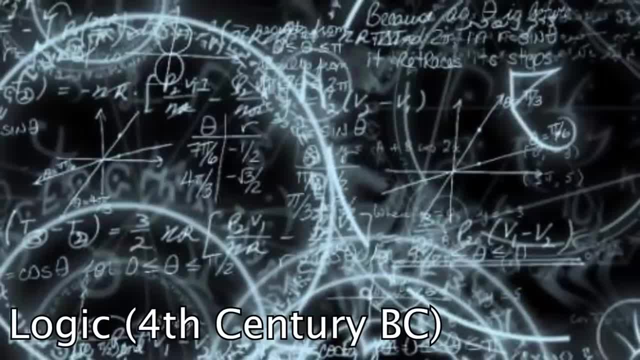 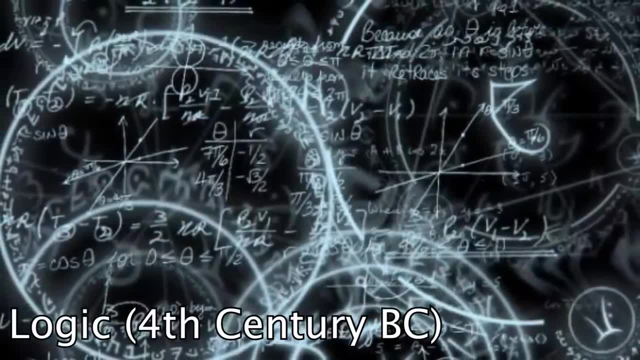 Although a lot of advancements in this field were done in the 19th and 20th century, it started around 2,500 years ago. In a logic class nowadays, you'll notice some odd examples of problems that involve just thinking. For example, take the sentence: if it is raining, then the ground is wet. 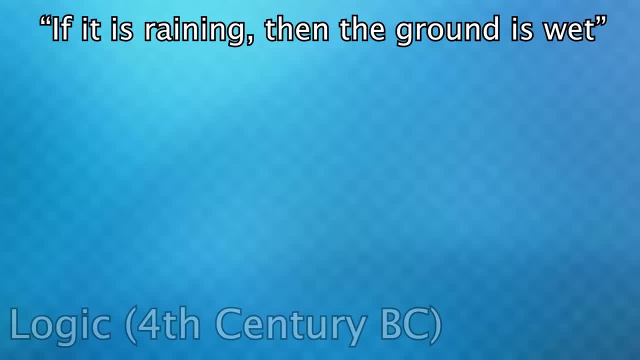 Let's say that is definitely a true statement. Now is this next statement also true: If the ground is not wet, then it is not raining. Anyone who's learned basic logic, which even includes various geometry students, can answer this in a second. 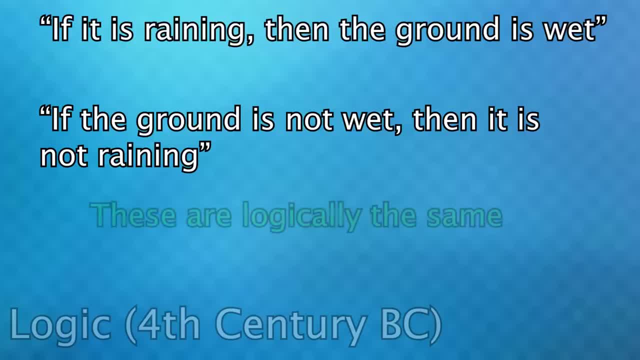 Others may need a little more time, but these two statements are, in fact, logically the same. In fact, whenever you say if something, then something else, it is always the same as saying: if not the second thing, then not the first thing. 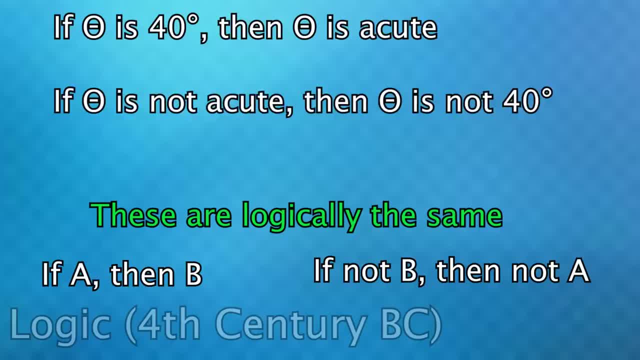 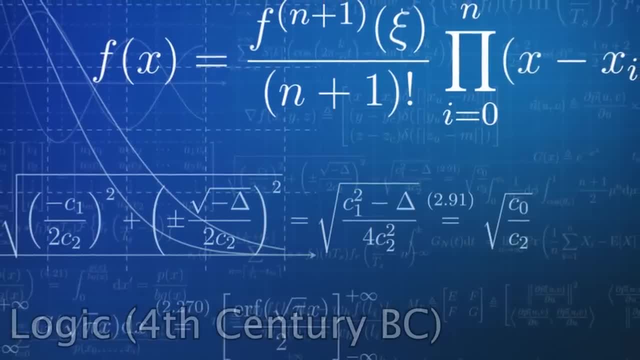 If an angle is 40 degrees, then it is acute, and if an angle is not acute, then it is not. 40 degrees are logically the same thing. Concepts like this may seem weird, but within mathematics we need very formal language that we all agree on. 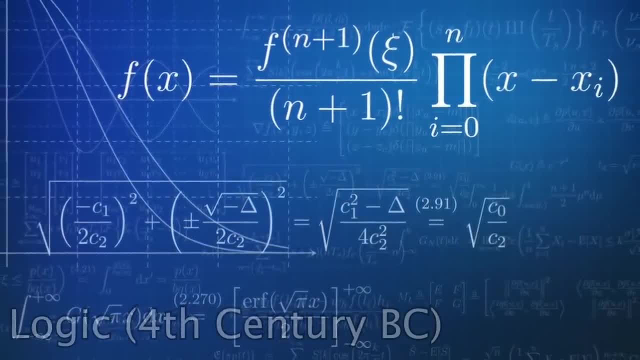 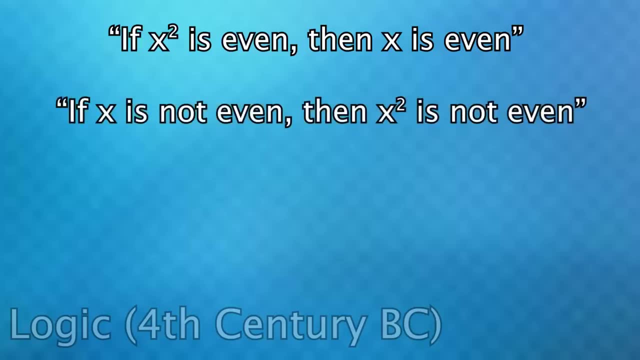 in order to prove theorems that are extremely difficult to understand. If you were asked to prove the statement if x squared is even, then x is even, you now know you could also prove: if x is not, even, then x squared is not even. 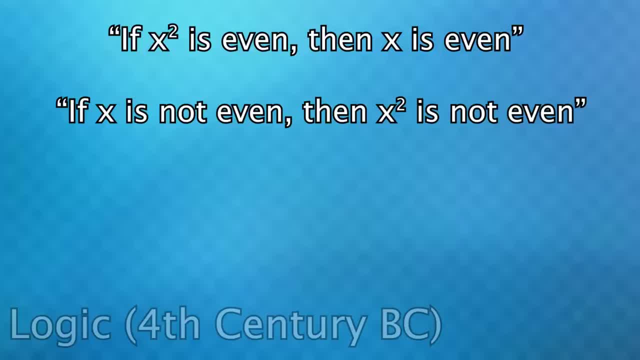 Proving one automatically proves the other and, although this is an easy example, when dealing with more advanced mathematics we need a very clear understanding of the language and logic behind every statement. Then, a little later, just over 2000 years ago, 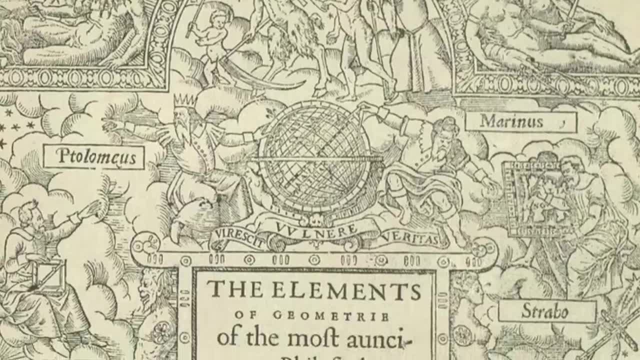 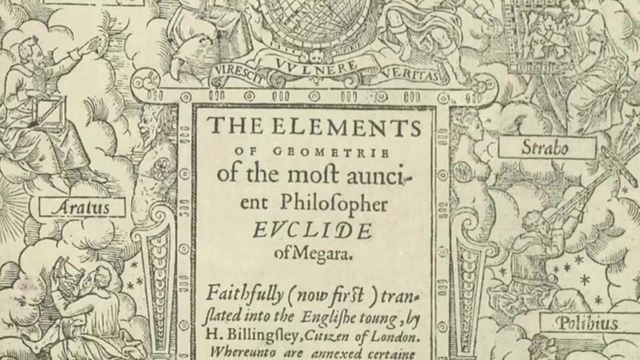 the mathematician Euclid published a series of 13 books known as Elements, which many regard as the most influential textbook of all time. While there is a lot discussed in these books, one important concept is the Euclidean algorithm, or Euclid's algorithm. 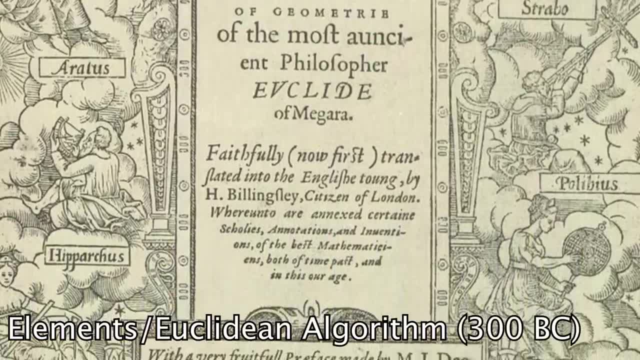 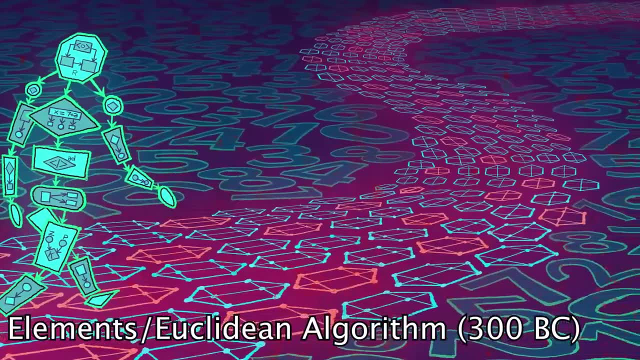 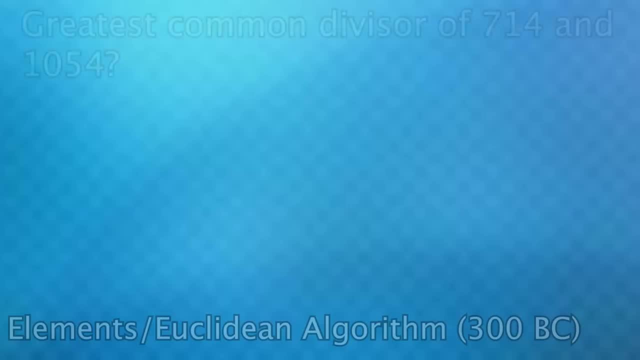 one of the first mathematical algorithms ever discovered. An algorithm is simply a series of steps that solves a problem, executed often, but not always, by a computer. This algorithm calculates the greatest common divisor of two numbers in an efficient way. So if you want to know the largest number that goes into, let's say, 714 and 1054,. 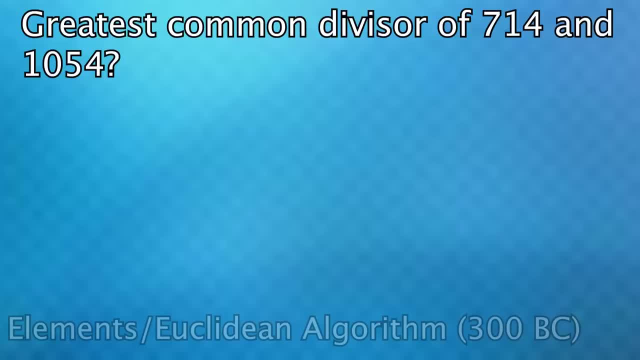 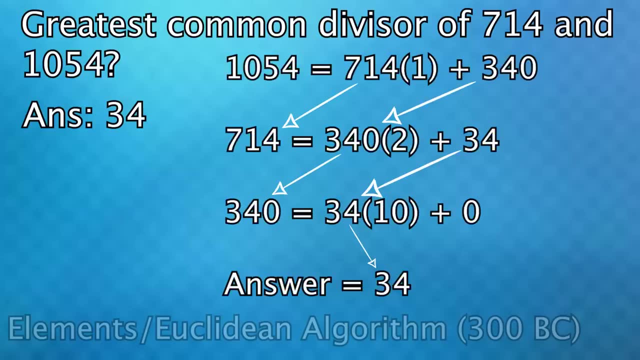 it would not be that hard but may take a little bit of time to find the answers 34.. Instead, we can use the algorithm. I'm not going to explain how it works, but it just involves basic elementary equations and elementary school arithmetic. 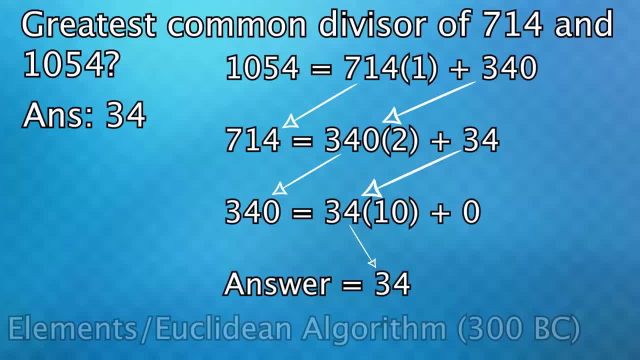 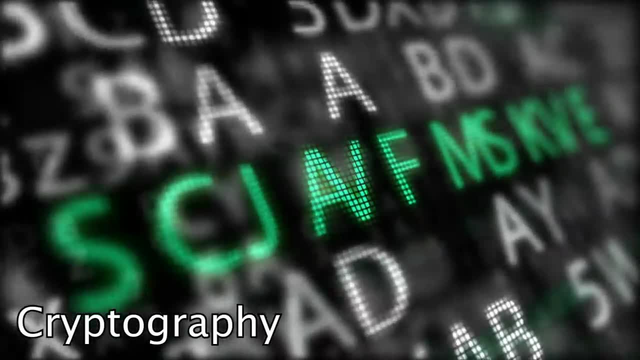 and using it, you can probably figure out the answer by hand in less than a minute. I mention this algorithm because it extends to the field of cryptography. Cryptography is really about techniques that ensure secure communication, especially in the presence of adversaries such as hackers. 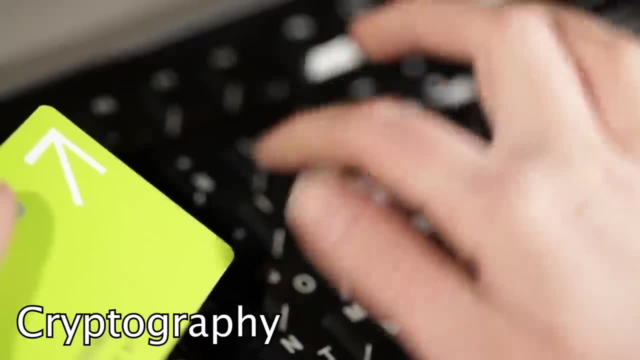 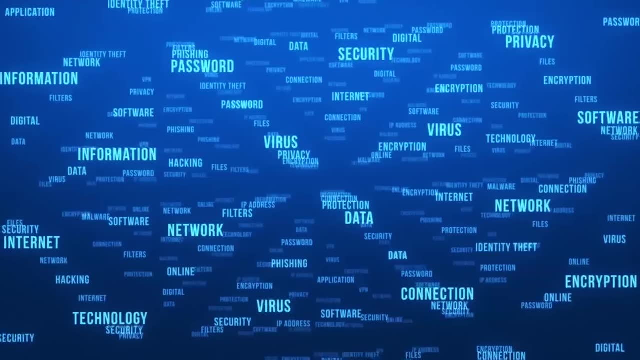 When putting sensitive information online. let's say, normal text is encrypted using mathematical techniques that turn it into text that cannot be understood by a third party or really anyone, at least until it is decrypted back to original text, which you need a secret key to do. 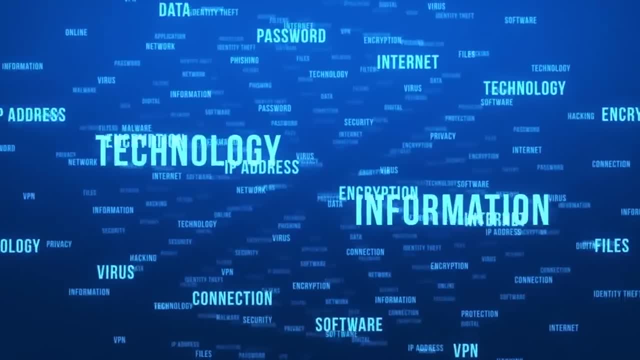 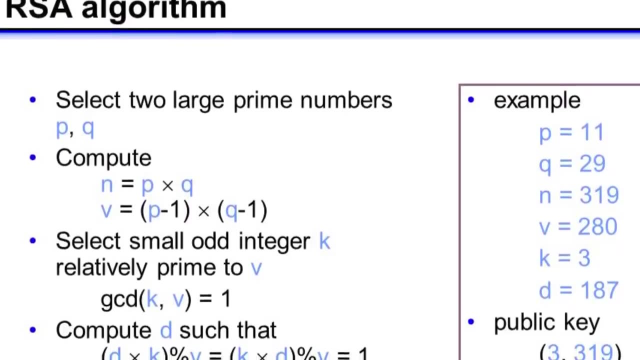 that only the receiving party should have. Although there are various methods of encryption, certain types, such as RSA, rely on the fact that it is very difficult to break large numbers up into prime factors. Cryptography heavily involves number theory or the study of integers. 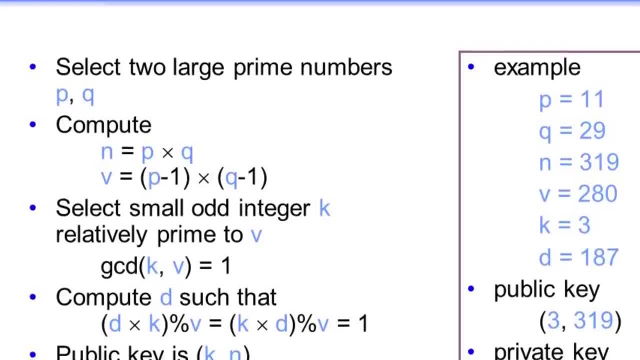 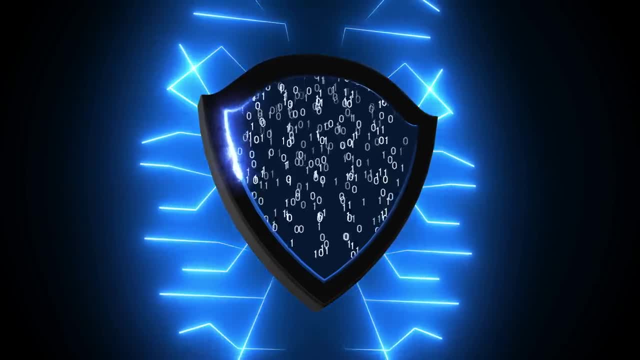 which is why that Euclidean algorithm from before has applications in this field. This is what protects our passwords, credit card numbers and any type of sensitive online information. In fact, the NSA, or National Securities Agency, is the largest employer of mathematicians in the United States. 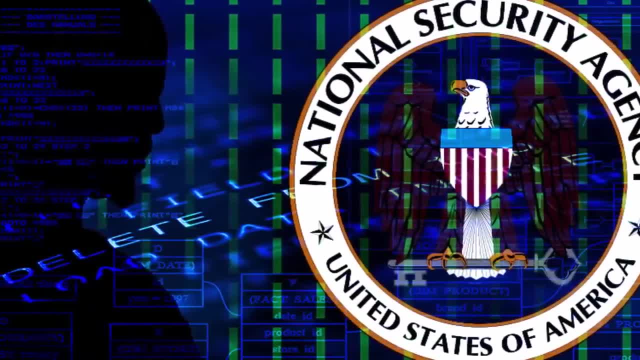 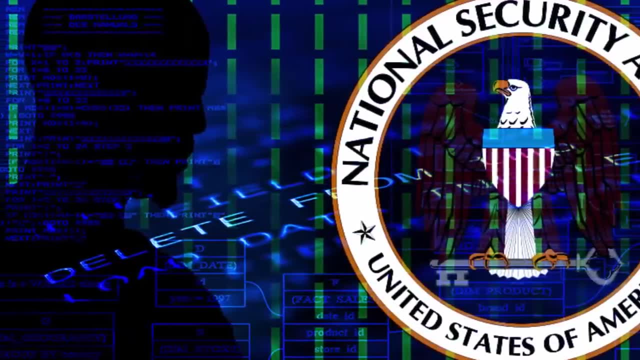 as they need those mathematicians to create and break these codes. You may think cryptography is a recent development, as computers have not been around for even a century yet. However, it dates back hundreds of years where written letters were encrypted for privacy purposes. In fact, techniques to decipher these encrypted messages. 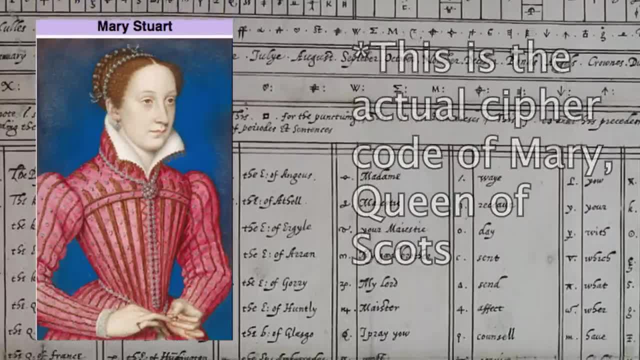 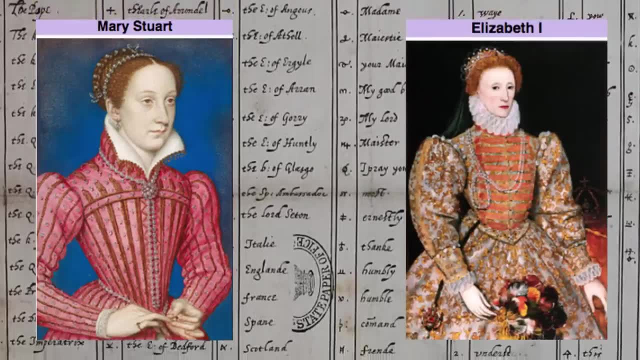 were used on messages from Mary, Queen of Scots, which revealed that she had sanctioned an attempted assassination of Queen Elizabeth, and she was executed shortly after that, in 1587.. Moving on, there were, of course, several hundred years of discoveries that we all know of very well. 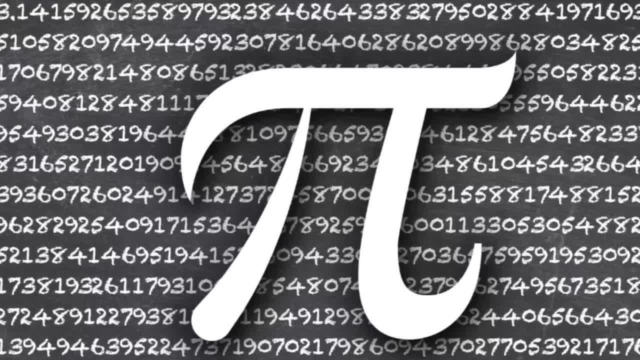 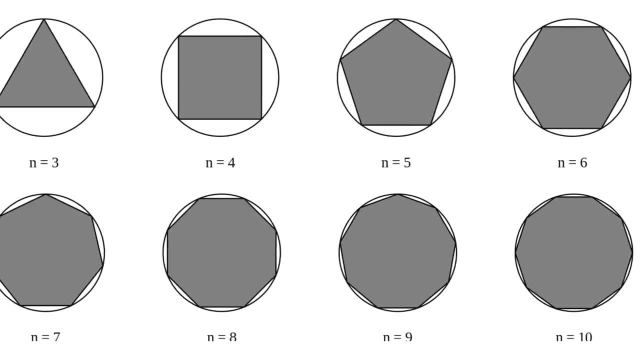 For example, the discovery of pi, which actually took a lot of work to pinpoint exactly. It was approximated as 3.125 and also 3.16 for a while, until several years later better approximations were made Then: logarithms, geometry, algebra, basic Cartesian coordinates. 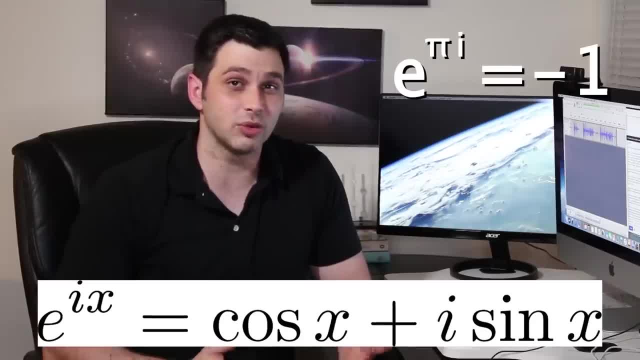 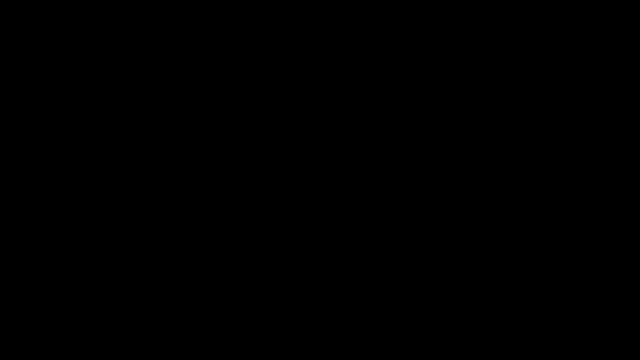 and complex numbers which I made an entire video on and so on, were all discovered hundreds to even thousands of years ago. so I'm not going to cover those in any detail. But if you want a random fun fact, the radius of the Earth was approximated in the 3rd century BC. 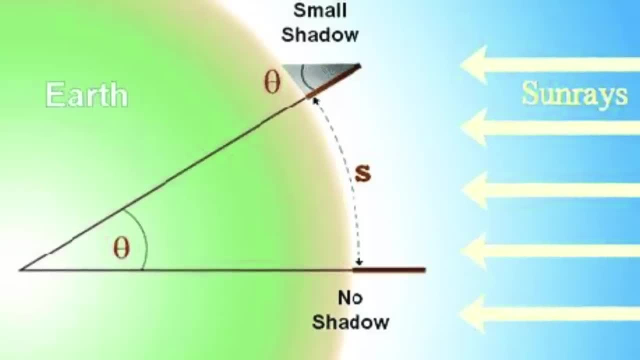 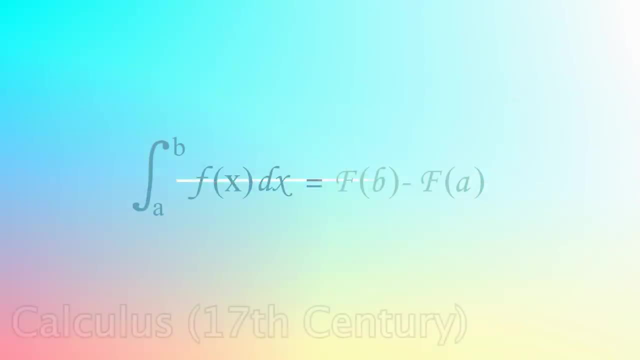 to nearly 99% accuracy, using basic geometry, deductive reasoning and just measuring a shadow length. But with that said, now I'm going to jump ahead to the 17th century, when calculus was introduced to the world, which would change math and physics forever. 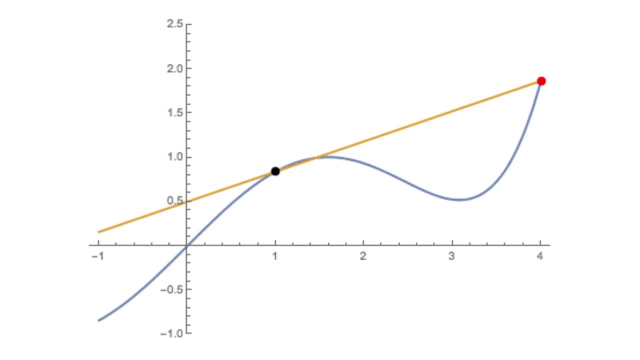 Newton was concerned with analyzing rates of change, not as an average, like average slope, but at one instant. This instant rate of change became known as a derivative, telling us that change in some parameter with respect to another at, again, one specific instant. 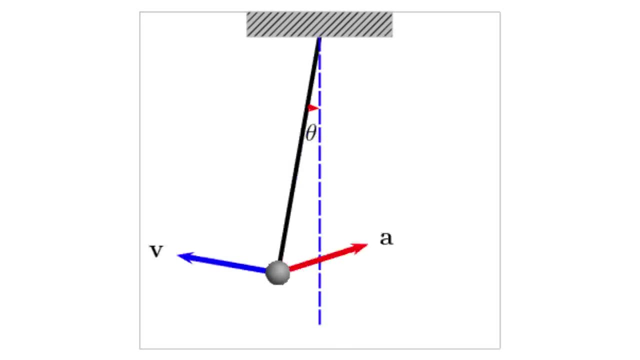 For example, if your speed is constantly changing, algebra can tell you the average speed, but calculus can tell you the exact speed at any moment in time, kind of like what a radar gun would read. This gave us much more powerful insights into the motion of planets. 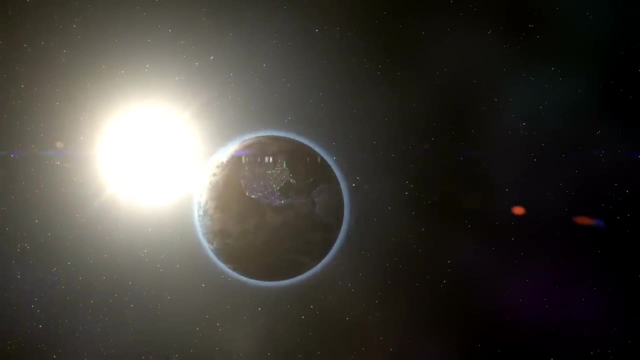 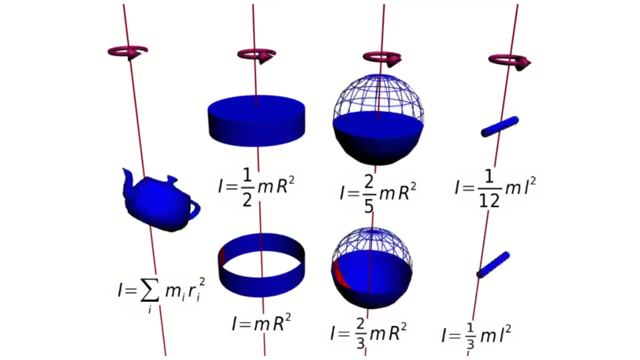 and how they change their speed throughout an orbit. Then the motion and behavior of electromagnetic waves is expressed through calculus. moment of inertia, or essentially an object's resistance to rotation, is calculated using calculus techniques, and calculating the work done on a particle moving through a complex vector field requires calculus. 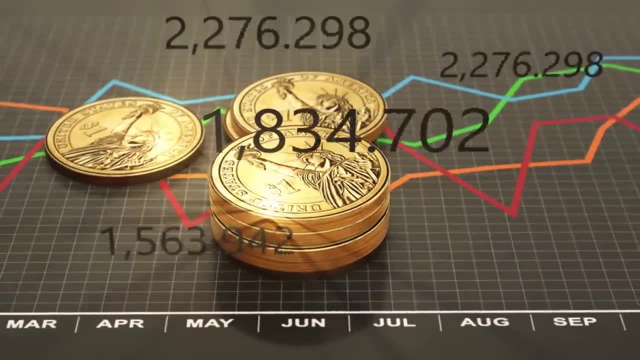 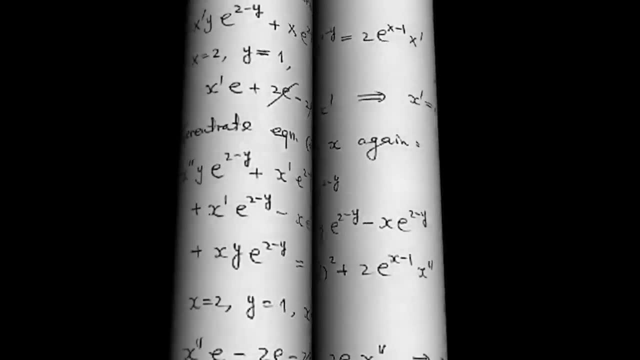 Calculus is used within economics and maximizing profit, chemistry and calculating diffusion rates and so much more. There's no way to do justice for all the applications of calculus, but whether you study engineering, physics, math, chemistry, bio or even business in college, 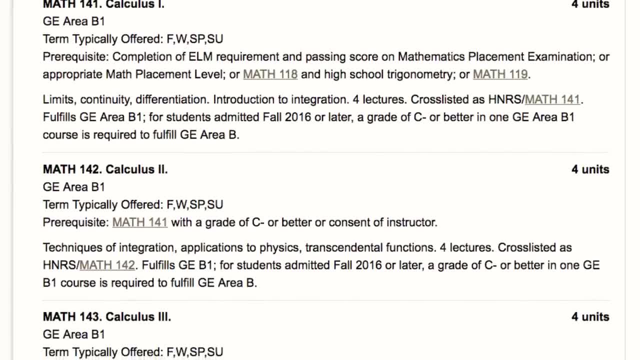 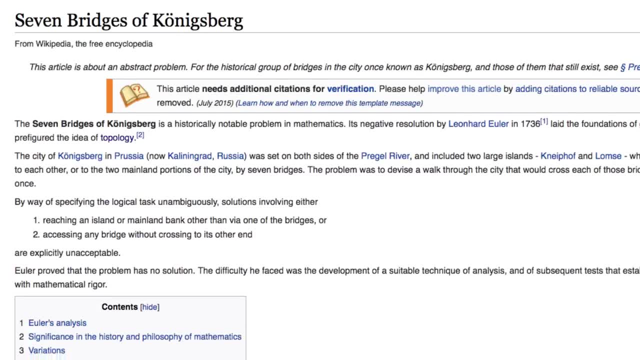 unless you have all the needed credits, college will start with a series of calculus courses to be used later on. Next, in 1736, Leonard Euler published a paper on the Seven Bridges of Konigsberg, which is regarded as the first paper in graph theory. 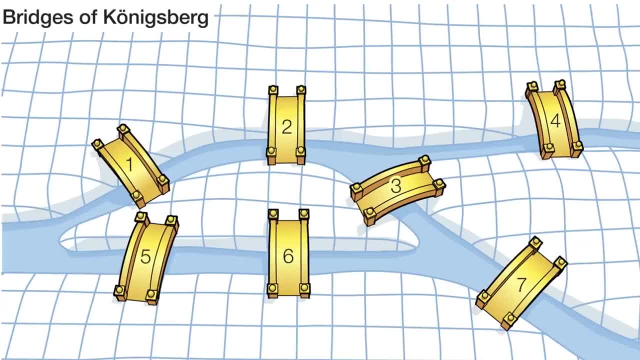 The question was quite simple: Given this network of bridges, can you cross each bridge exactly once, of course without going into the water? You can try it for yourself, but spoiler Euler eventually proved it to be impossible. Graph theory is not about the graphs you know from middle school and high school. 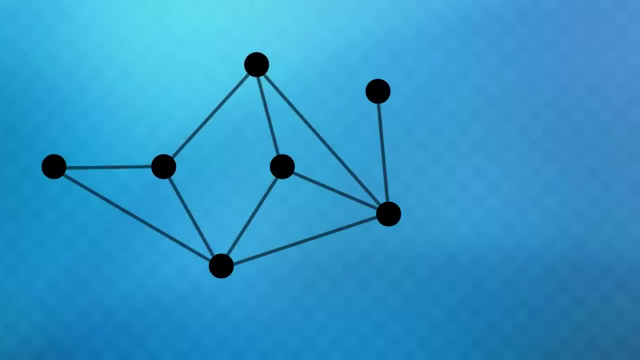 A graph here is made up of nodes and edges that connect them. This could have a wide variety of applications, many of which lie in the field of computer science. A graph could have nodes that represent people and their connections could represent compatibility, in which dating sites need to use algorithms to create best matches. 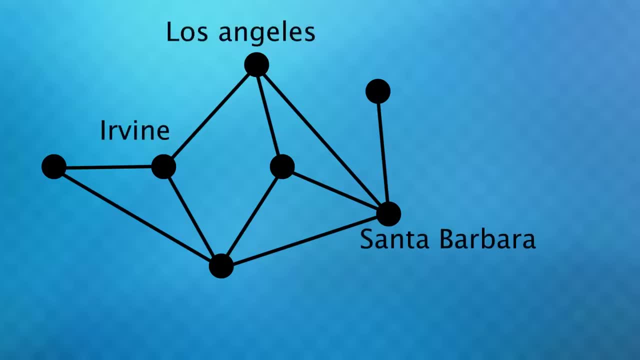 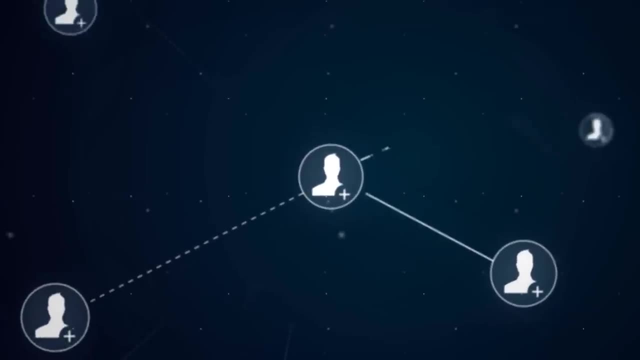 Nodes could be cities and edges are routes that connect them, where you need to figure out the shortest path from one point to another. Or a graph could represent how we are all connected through social media or another social structure. This investigation is known as social network analysis. 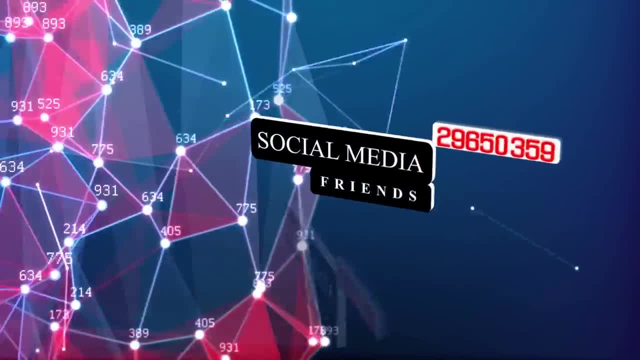 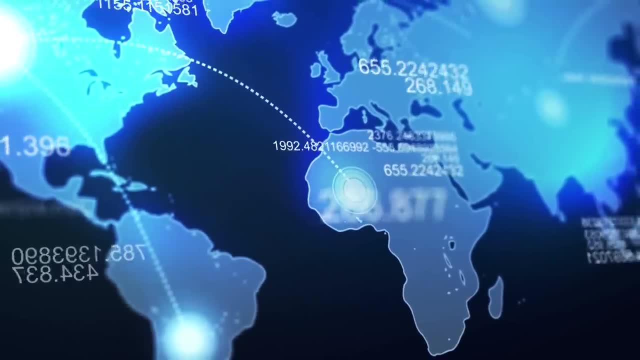 which is used, for example, in security applications to map out information on street gangs, terrorist organizations and more. To end this subfield and emphasize how powerful graph theory can be, it has made two computer science graduates, Larry Page and Sergey Brin, billions of dollars. 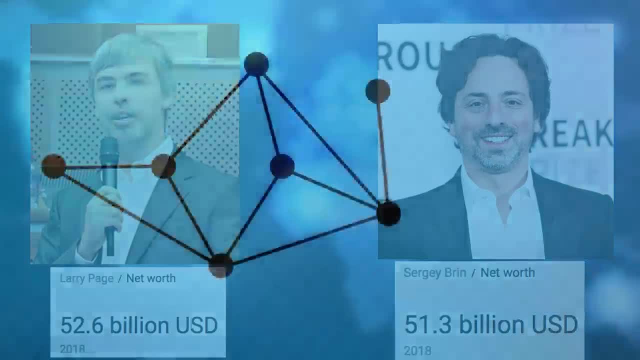 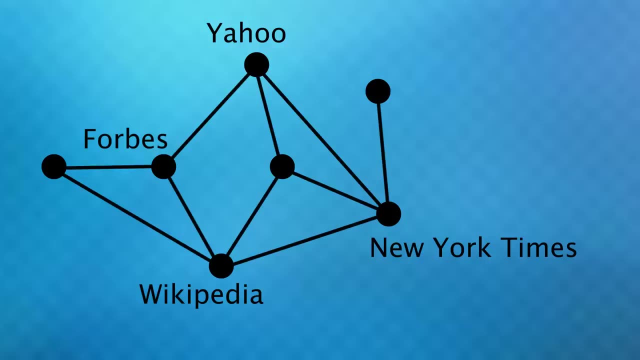 In the 90s they used graph theory in such a way that nodes represented websites on the internet and if one website linked to another, that would be represented by an edge. The more links going to a website, the quote, better that web page would be considered. 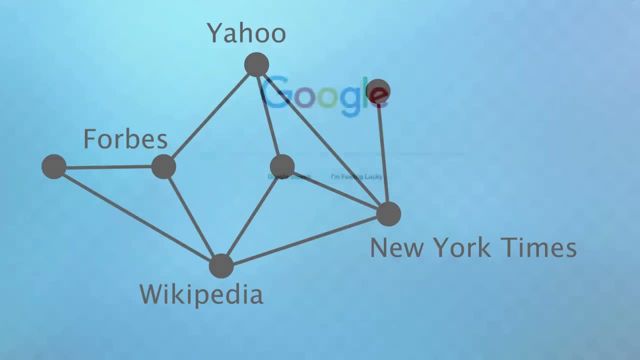 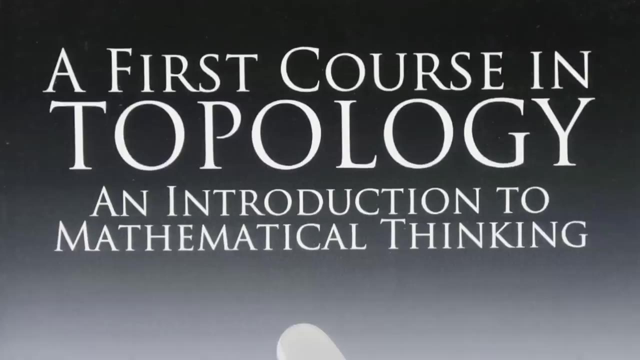 This algorithm to rank web pages became the backbone of what is now Google. Out of Euler's seven bridges of Konigsberg paper not only came graph theory, but also the field of topology, one of the most advanced math courses you would take if you studied math as an undergrad. 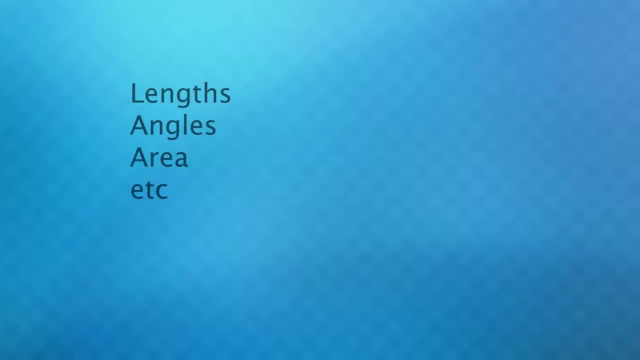 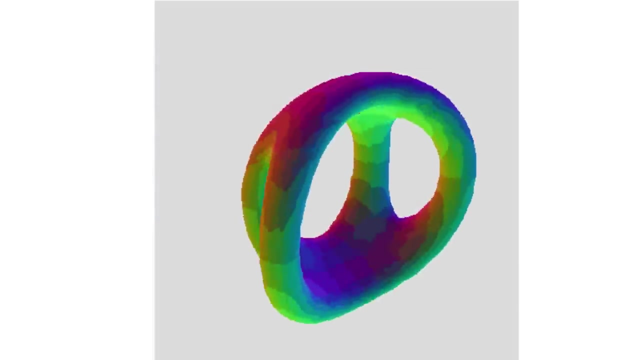 In topology, you have to forget about the notion of lengths and angles, like in geometry. In this field, you care more about connectedness and holes, for example, where bending and stretching is totally fine and does not change the properties of the space that we care about. 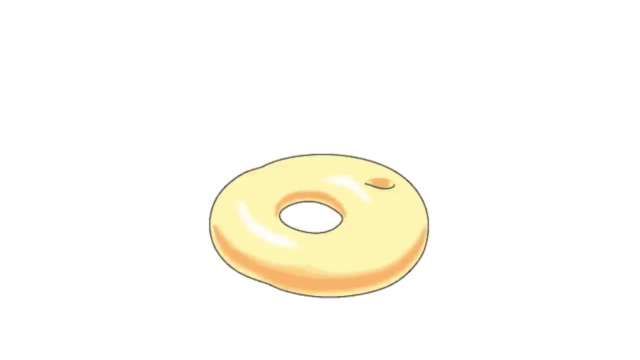 For this reason, in topology they famously say that a donut and a coffee mug are the same thing. The questions of can you morph one object into another or whether the two are homeomorphic is important. within topology, You'll analyze complex shapes, higher dimensional objects, knots and so on. 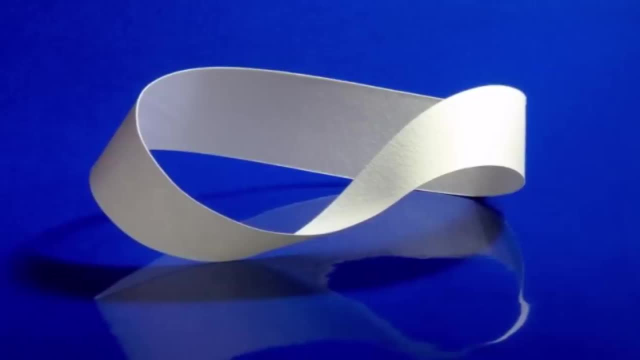 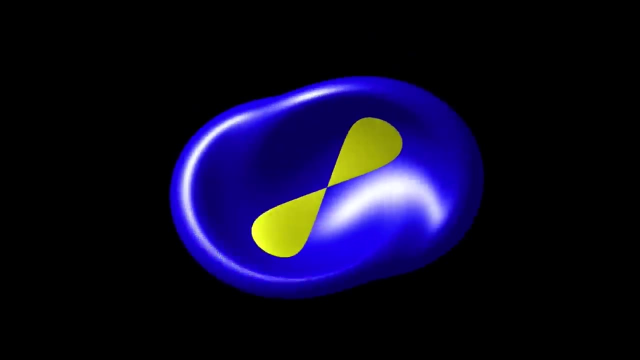 This class allows you to understand the mathematics of things like cutting a mobius strip in half, which I did in a previous video, Or it reveals mathematically how you can turn a sphere inside out without cutting or tearing it or making any creases. while, yes, allowing self-intersections. 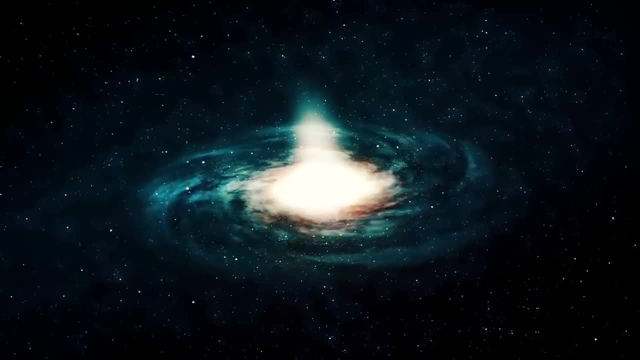 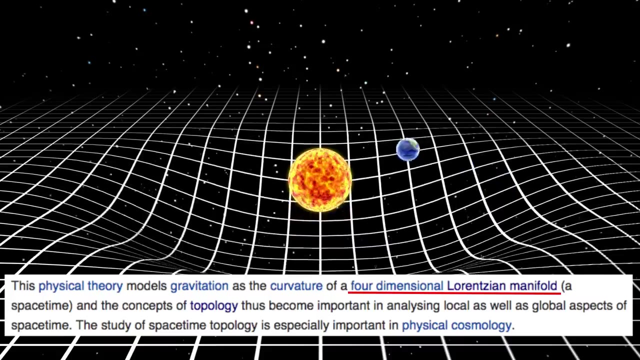 Topology applies to fields of physics such as quantum field theory or cosmology In general. relativity states that space-time is a four-dimensional Lorentzian manifold, and analyzing this involves concepts within topology. In robotics and motion planning, all the possible states that the robot can be in. 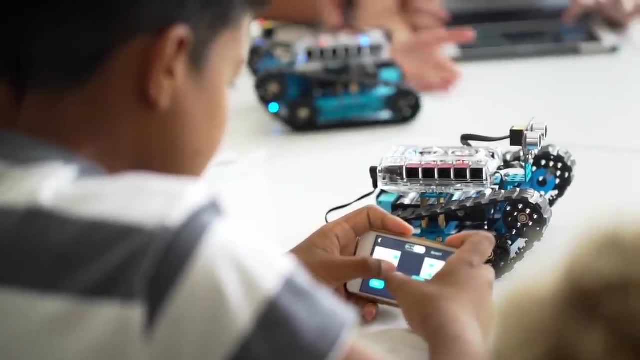 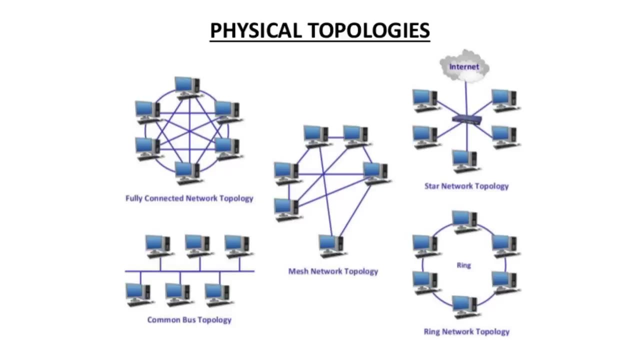 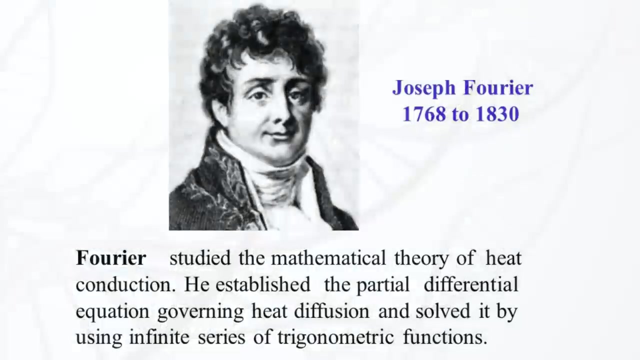 or the configuration space can be modeled using concepts taught in topology. In computer science, topology can be used to model how networks are connected and how data flows, And even knot theory is used in biology to analyze how enzymes cut and reconnect DNA. Next up, in 1822, Joseph Fourier published a paper. 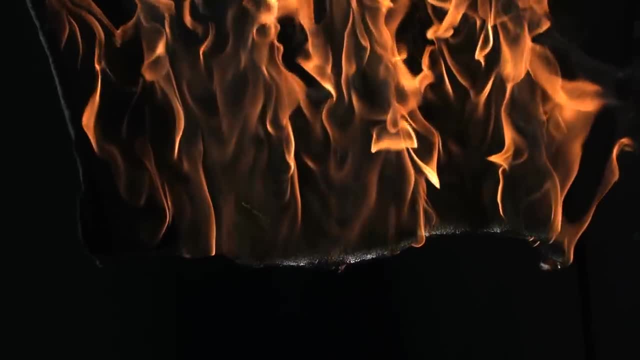 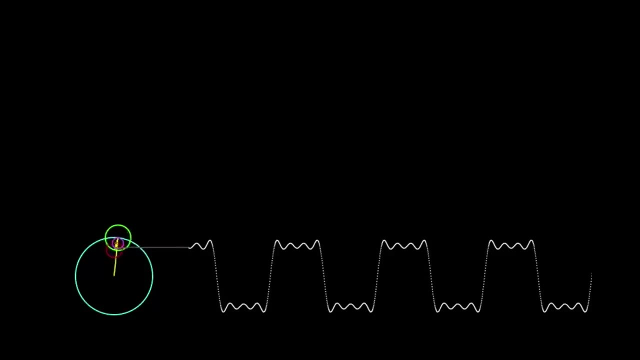 on heat flow, and while working on that he made a discovery that would go on to have a wide range of applications. This discovery we now call the Fourier transform. He determined that any function, no matter how weird it looked, could be broken up into just a sum of sine and cosine functions. 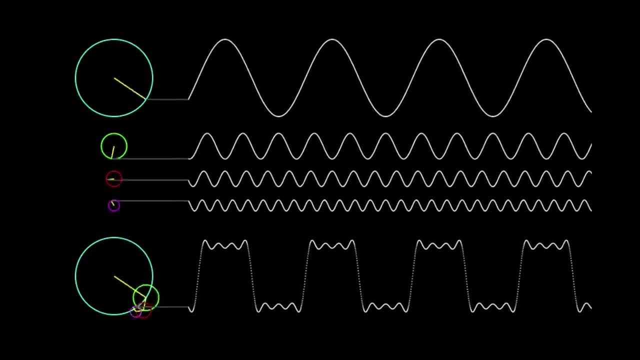 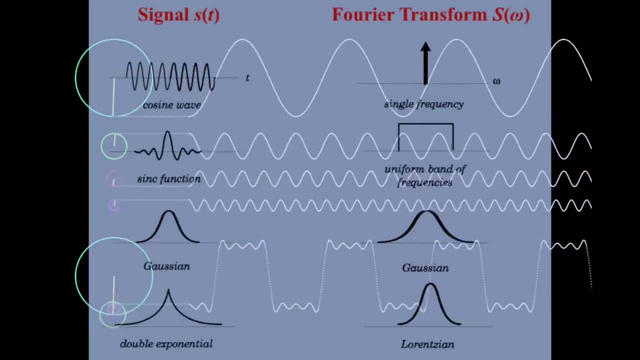 As in: if you just take a bunch of these sine and cosine functions and pick just the right frequencies and amplitudes, you could add them up to make any function you wanted. This has lots of applications, but the main ones are in quantum mechanics and signal processing. 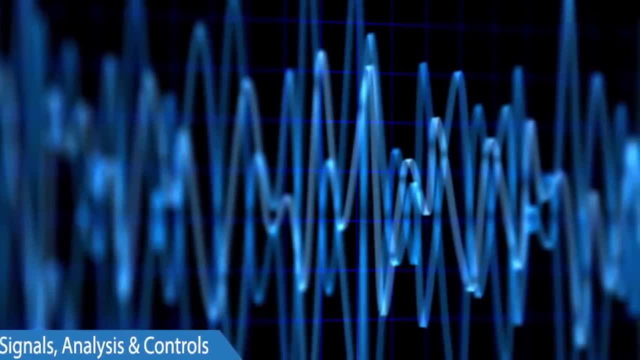 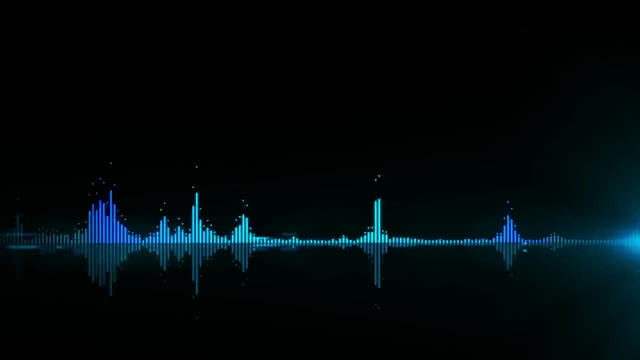 When looking at real-world signals, whether it be a radar signal, a signal from a digital image, sound or even light- the physical signal itself can be quite complicated and not tell us much. By using Fourier analysis, we can break that signal up into those trig functions that make up the signal in question. 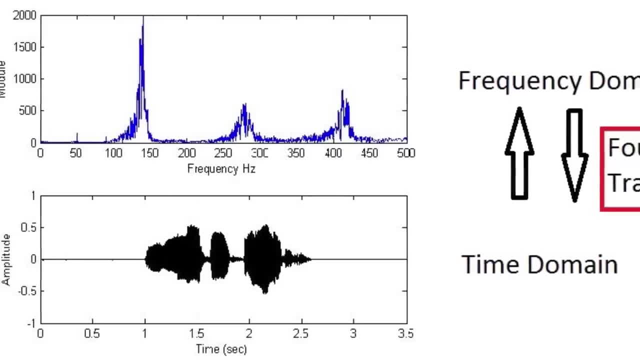 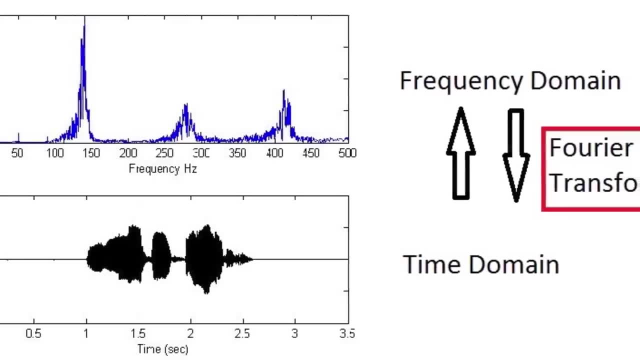 which reveal properties that cannot visually be seen originally, Like whether the signal is made up of much higher frequency sources or lower frequency sources. Then, although difficult to trace back to a specific date, the fundamentals of a field known as group theory began in the early 1800s. 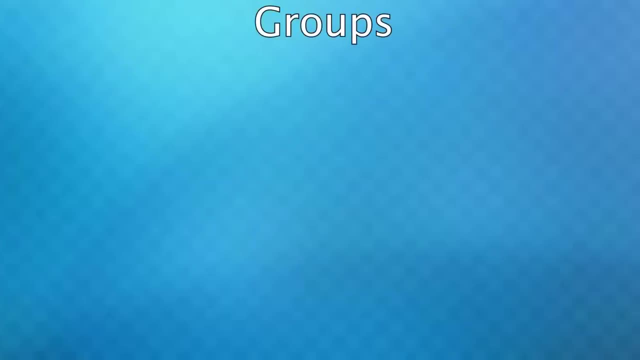 This is all about the study of groups, and a group is basically a set of elements that, along with some operation, satisfy certain conditions. The set of integers under addition is a group. for this reason, If you pick any two integers and add them up, you get another integer, something that's in the set. 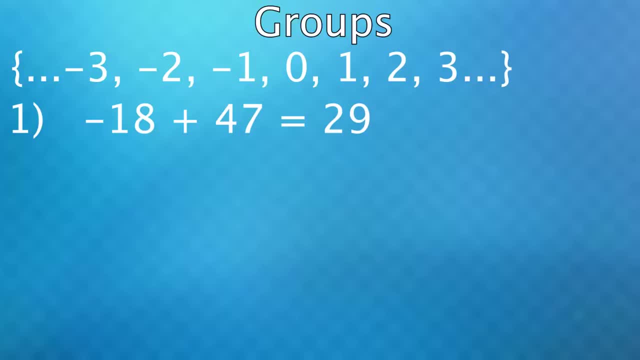 Then there also exists an integer in the set- in this case zero- where if you add any number in the set to it, you get the same thing out. Next, for any number in the set, there exists another, such that if you add them, you get that identity from before, which was zero in this case. 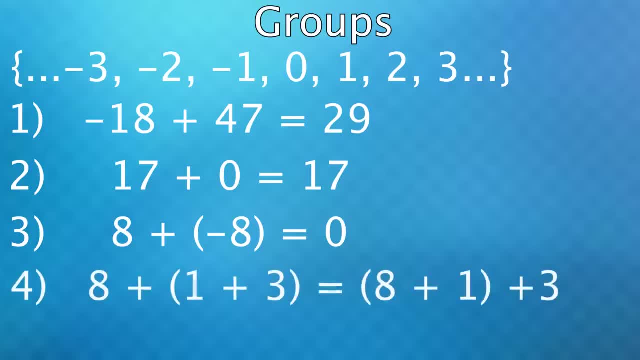 And lastly, how you group certain numbers under addition does not change the result. These four properties of closure, an identity element, an inverse element and associativity mean the set is a group. Yes, this seems very weird and random, but group theory has given us a lot of insight into the mathematics of symmetry. 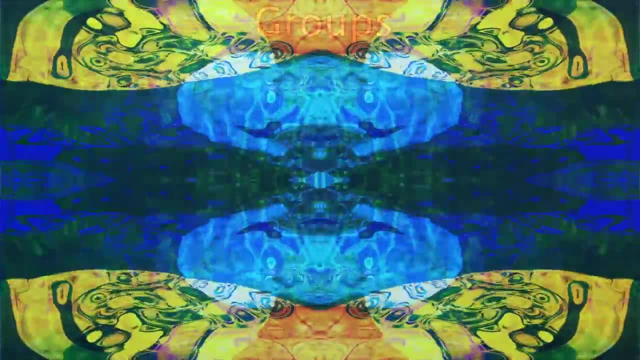 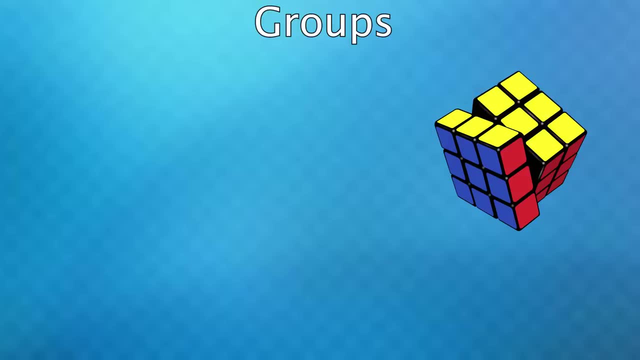 This math can apply to sets of numbers, but it applies to other sets, such as the manipulations of a Rubik's cube. All the ways that a Rubik's cube can be altered form a group with its own unique properties. In our last example, with integers and addition. 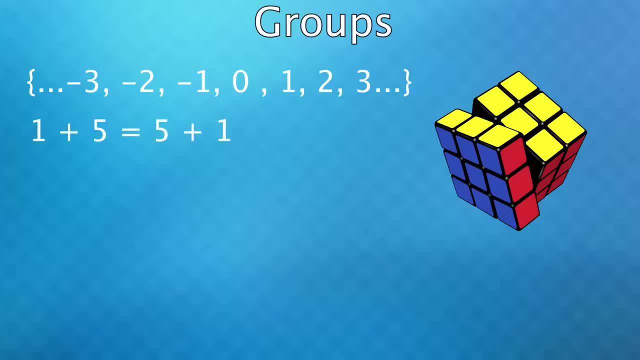 you can easily see that the order of the integers does not matter when you add them. The fact that you can swap two numbers and get the same result means the group is commutative, otherwise known as an abelian group. Knowing that is the group of all possible Rubik's cube manipulations. 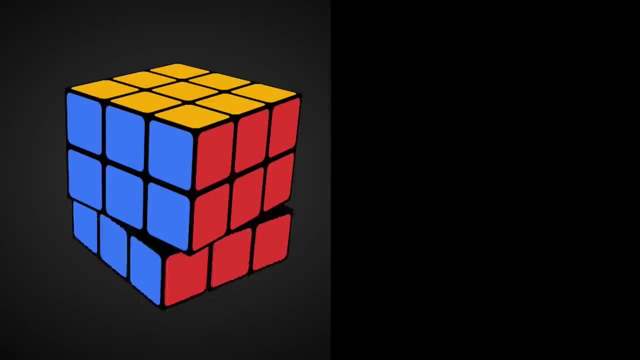 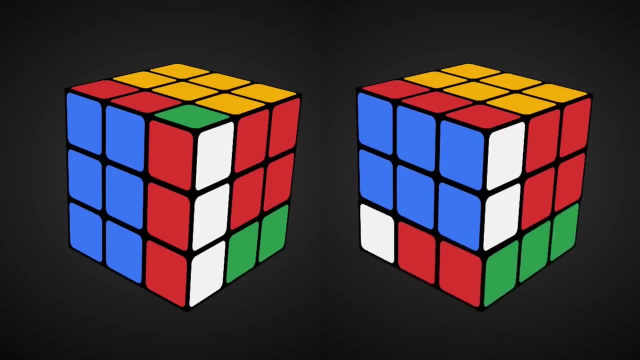 an abelian group, As in: if I turn the bottom 90 degrees, then the front face. is that the same thing as turning the front face and then the bottom? May take a little thought, but the answer is no. this is not an abelian group. 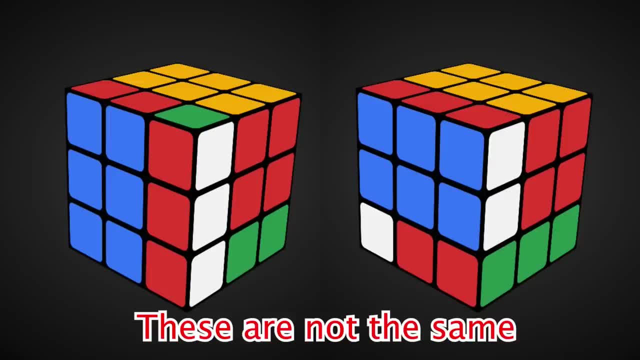 While you don't need group theory to solve a Rubik's cube, group theory does give you insight into the mathematics behind the Rubik's cube. This mathematics of symmetry has applications in chemistry, for example, as groups can classify certain crystal structures and symmetries within molecules. 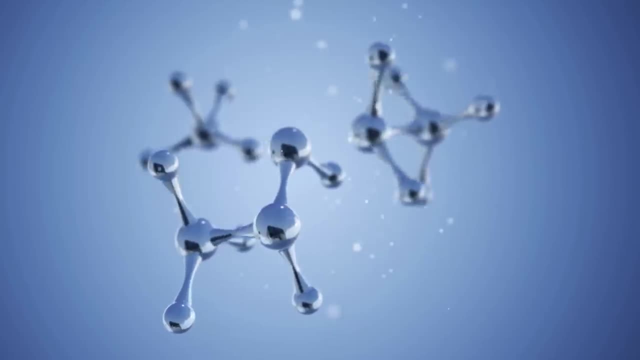 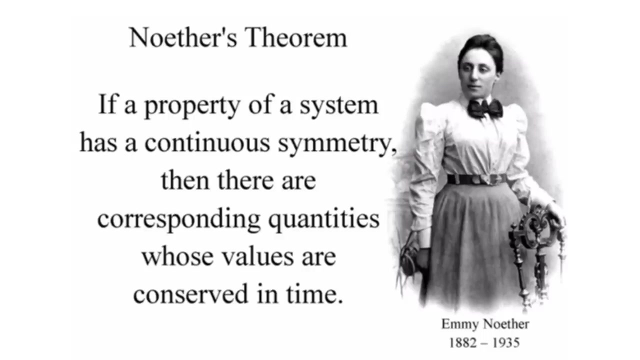 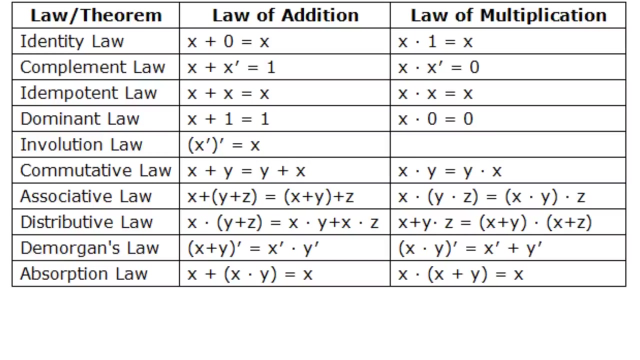 it can apply to public key cryptography and it has various applications in physics. For example, Noether's theorem explains how symmetry within a system corresponds to a conservation law, And this gave us a better understanding of Einstein's general theory of relativity. Then real quick: Boolean algebra, which was discovered in the 1800s. 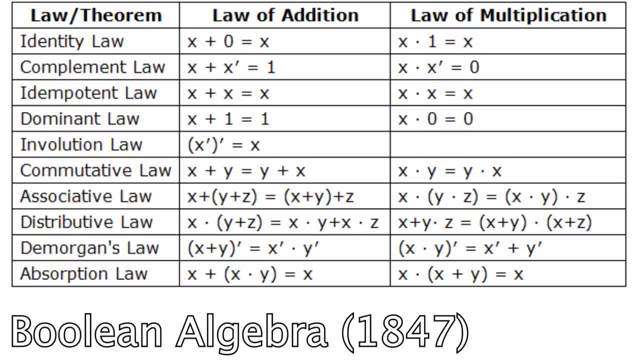 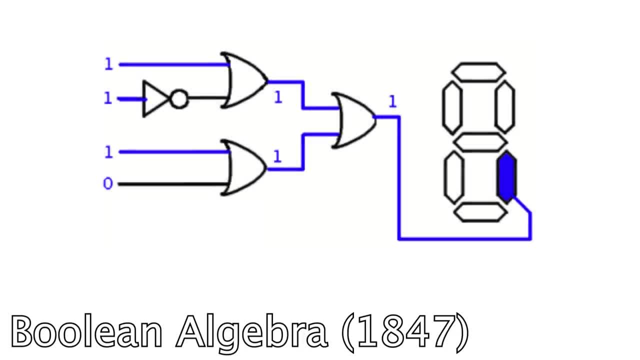 is essentially algebra using just ones and zeros, which can be used in computer applications. For example, using Boolean algebra you can simplify the amount of logic gates within a circuit, where these logic gates are what flip and transmit ones and zeros within a computer. The less of these there are, the faster a computer can run. 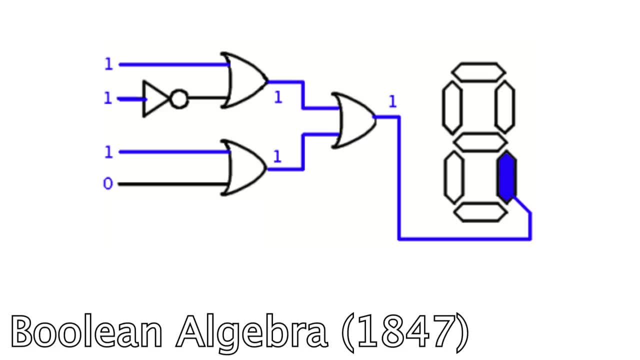 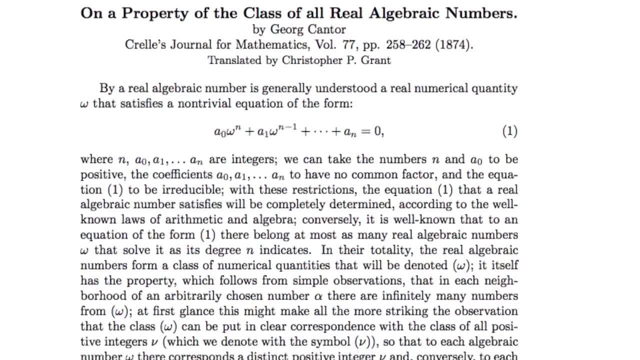 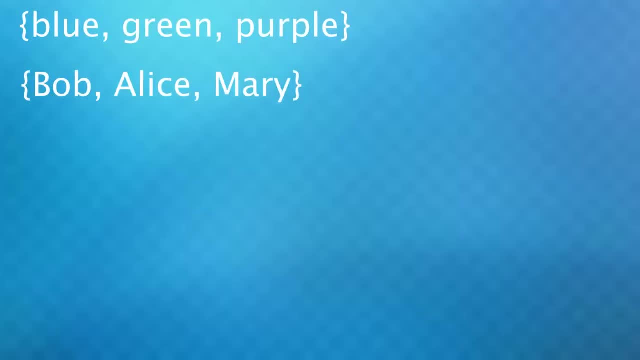 Moving on, in 1874, mathematician George Cantor published a paper titled On a Property of the Collection of All Real Algebraic Numbers, which is where the branch of math known as set theory began. A set is basically a collection of objects. it could be a set of colors, people, the set of prime numbers, even numbers, and so on. 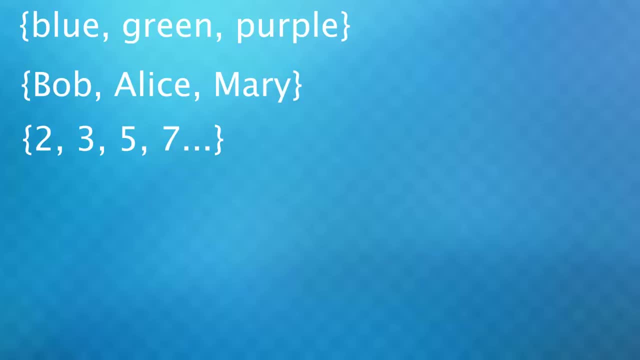 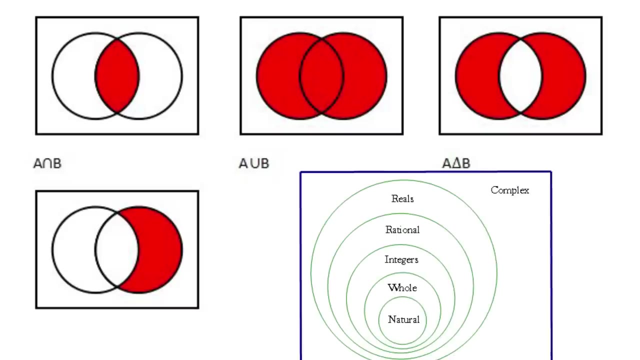 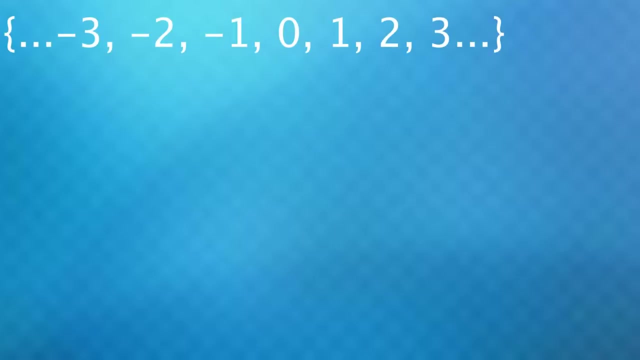 where each member is known as an element of the set. Set theory is concerned with the intersections of sets, unions, subsets or sets within sets, and what I'll cover now is whether a set is countable or not. For example, the set of all integers, which includes negatives, positives and zero, is countable. 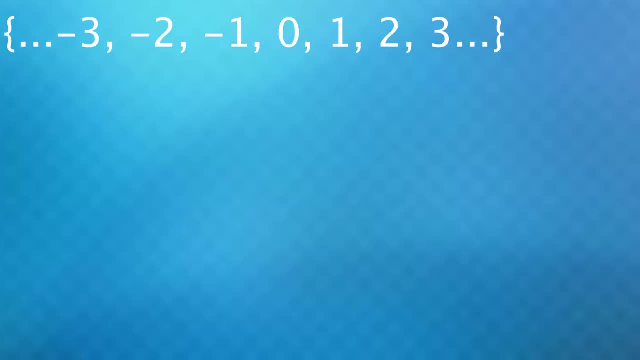 Now that does not mean that you can count every element in the set. It does go on forever and therefore is an infinite set, But it is countable, well, actually countably infinite, And that's because I can order all the elements such that nothing ever repeats. 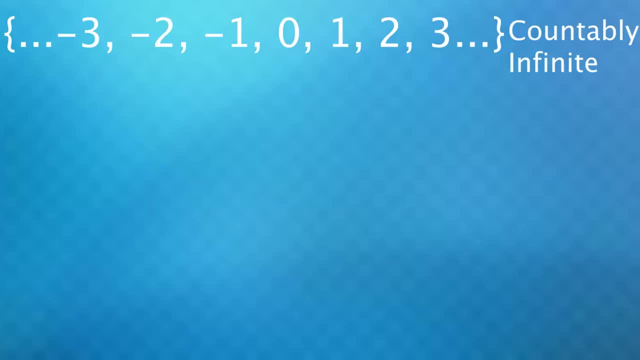 and I don't skip a number. I could put these in order such that I have zero, then one, then negative one, two, then negative two, three, then negative three, and so on. If I keep going, I would eventually hit any integer you could name. 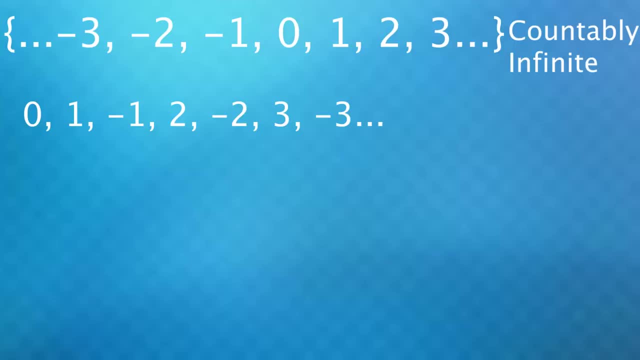 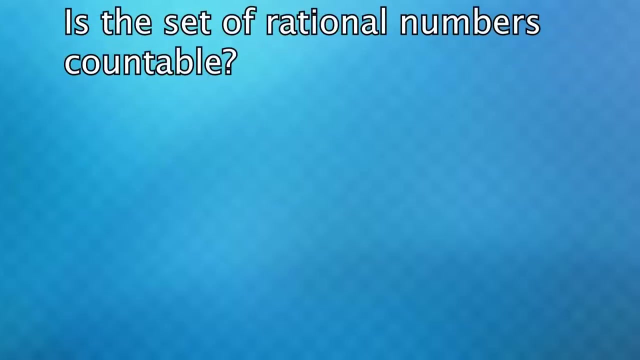 and I would not skip anything. Another way to think about this is: I can assign a natural number to every element of the set without skipping one. Now a tougher question is: is the set of rational numbers countable? Rational numbers are either decimals that end or decimals that go on forever. but repeat. 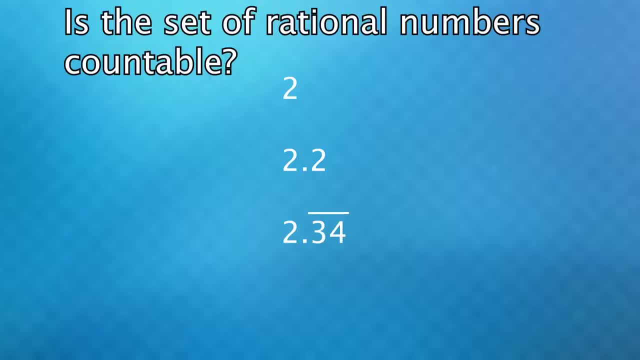 Two, 2.2,, 2.34, repeating 2.594, etc. These are all rational. Now could I line these up such that I have a first rational number, a second, a third and so on, such that I don't skip anything? 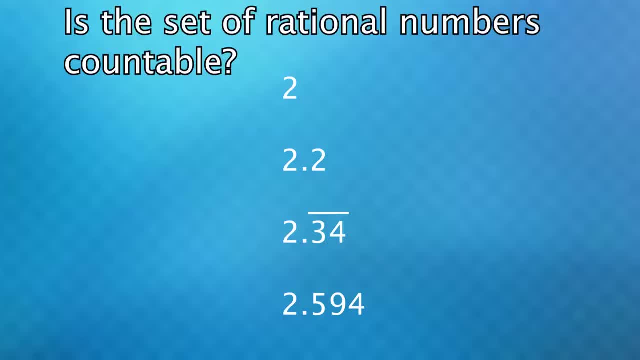 Amazingly, it was proved that the answer is yes. The set is countably infinite. First, remember that any rational number can be expressed as a ratio of two integers. Now, the most classic proof is ordering the rational numbers in a clever way, such that they are in this form: 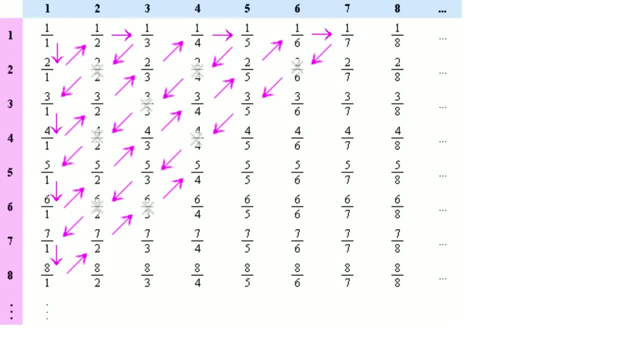 You have rows and columns of integers and every entry is the ratio of those two numbers. We can start at the top left corner where one is our first rational number, Then we go down to the next for the second, then diagonal, and keep going while skipping the rational numbers that repeat. 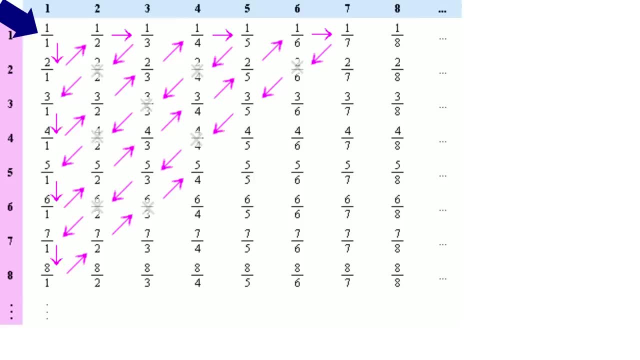 Doing this, we would eventually reach any rational number you could pick. Even this repeating decimal and therefore rational number is just 67 over 241.. And if you continued this pattern forever, you'd eventually find that 67 and 241 column and row. 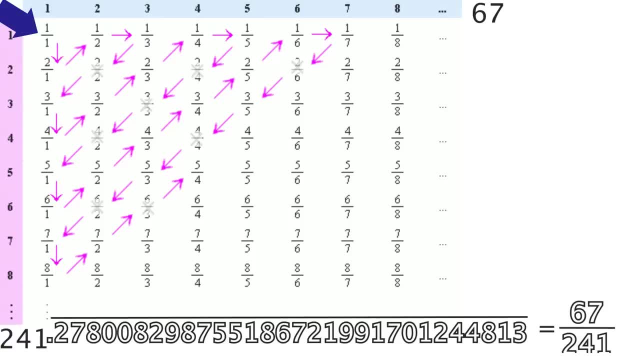 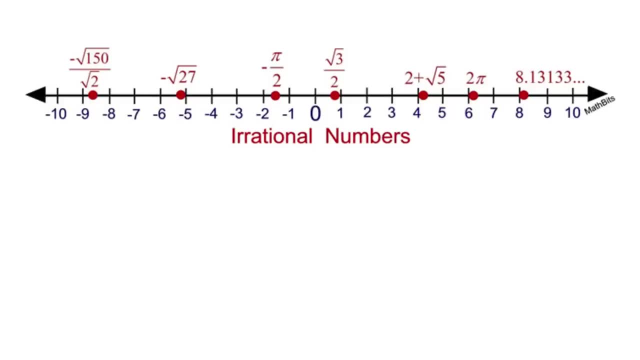 If you study math or maybe computer science in college, you will learn how the set of irrational numbers count. But the set of real numbers is actually not countable. There's no way to line them up such that you list every single one without skipping. 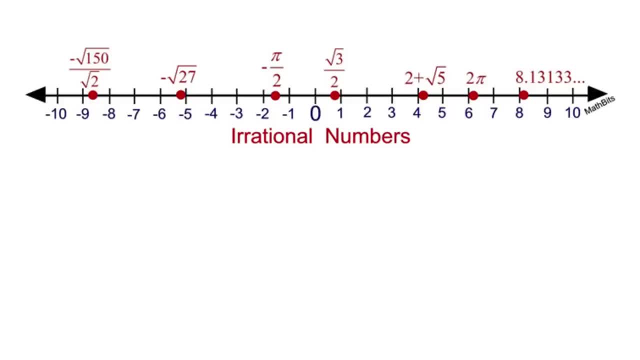 This means you could say that there are more irrational numbers than rational, even though there are an infinite amount of each. You'd also see that the set of real numbers, which includes integers, decimals, pi, square root of 2,, etc. is also not countable. 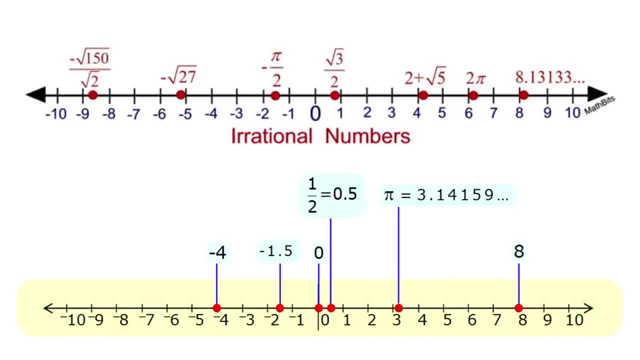 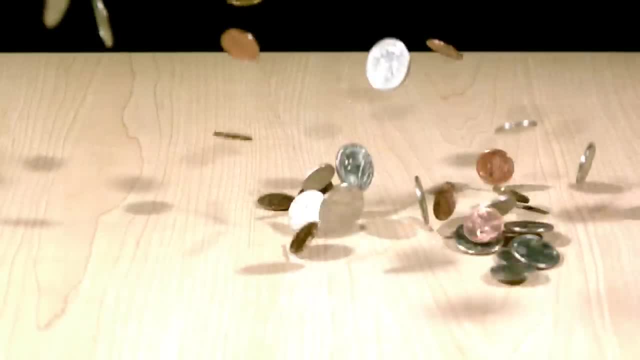 Set theory now has applications in several topics we talked about, including graph theory, topology, group theory and more. Now, when you flip a coin or play a game of roulette, every single event is an independent one. It does not matter what your last spin was. 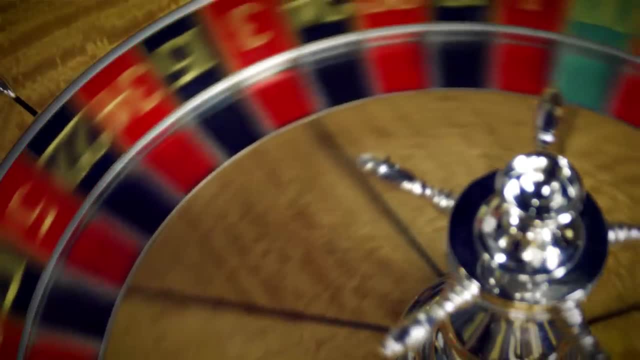 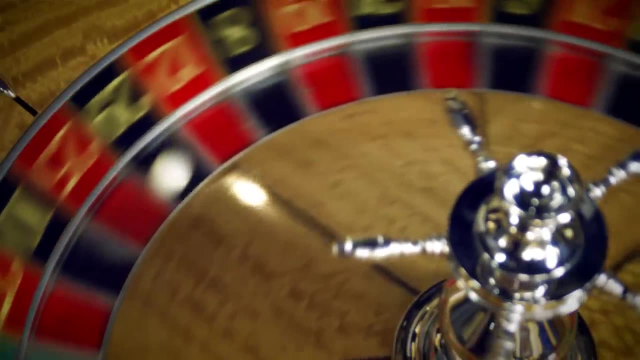 The odds of getting red on this next one are still the exact same as before. Well, in the early 1900s, work was done on a statistical model describing events in which probability depends only on the previous event. This model became known as a Markov chain. 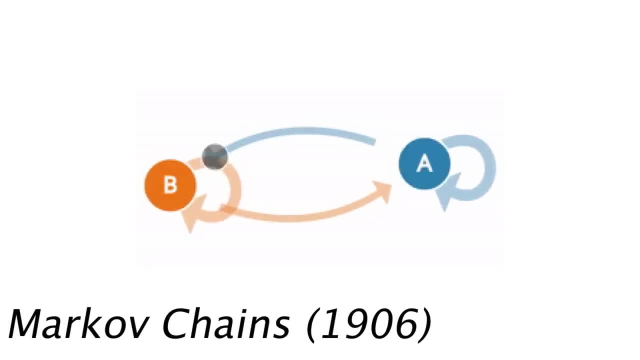 Markov chains include a state space and transition probabilities. Imagine you want to analyze the population of Los Angeles and New York. For simplicity we can say: people only can move from one to another or they can stay put. So maybe every year 10% of people who live in LA move to New York. 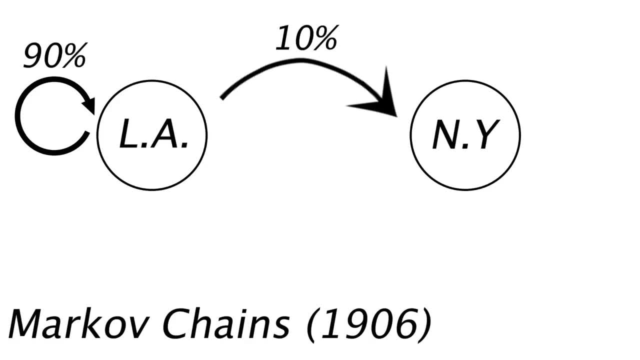 meaning that 90% of the people stay And, at the same time, every year, 15% of people in New York move to LA, meaning 85% stay. In this example, where you are now matters Based on if you're in LA or New York, we can predict whether a person may move or not. 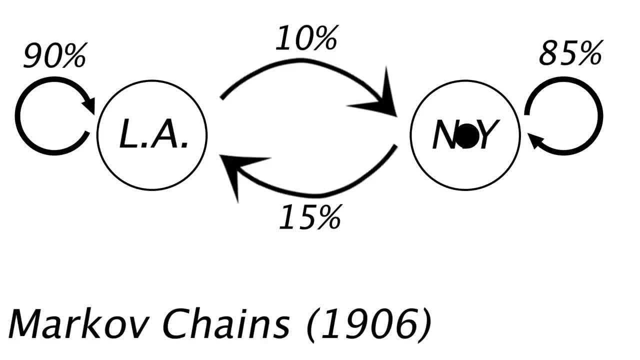 But saying that a person took this specific series of moves really does not matter in terms of what comes next. Using certain techniques, in this case linear algebra, you can determine how the system will evolve over time and whether it will reach some steady state or not. 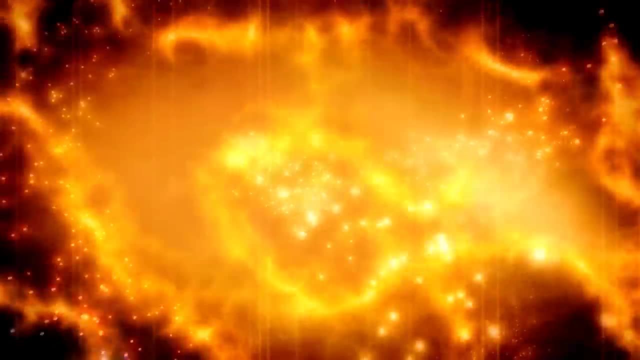 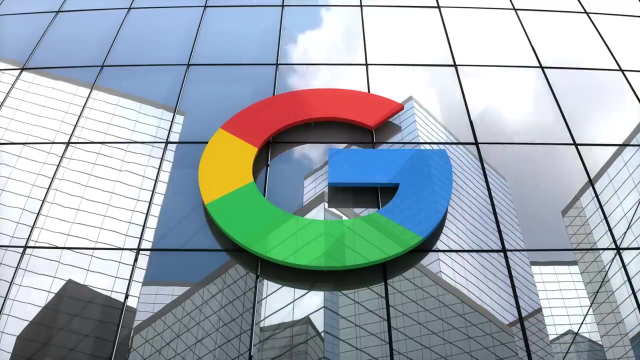 These apply to thermodynamics and representing certain unknown details of a system. they apply to modern speech recognition systems and they are what defines the page rank of a website, as used by Google. Then also, in the early 1900s, work was being done on the existence of a strategy. 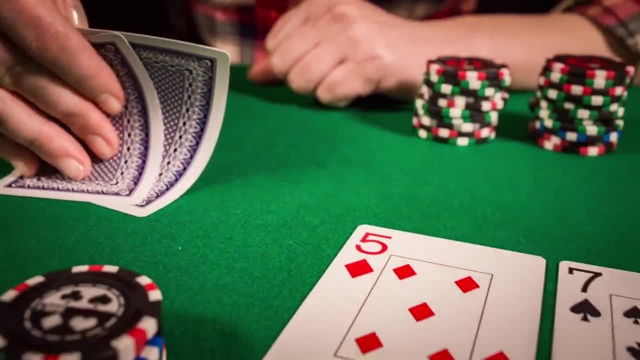 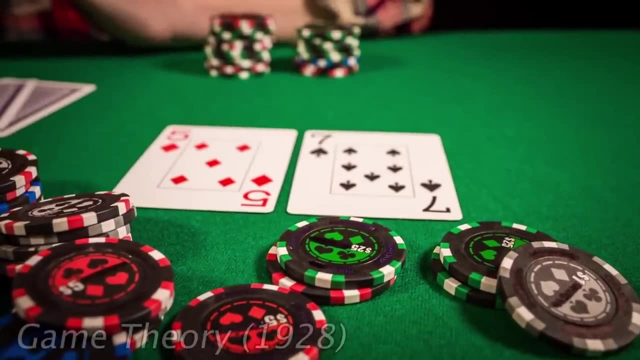 in two-person zero-sum games or games in which one person's gain is balanced out by another's loss. This field, started by John von Neumann in 1928, became known as game theory and quickly expanded throughout the mid-1900s. 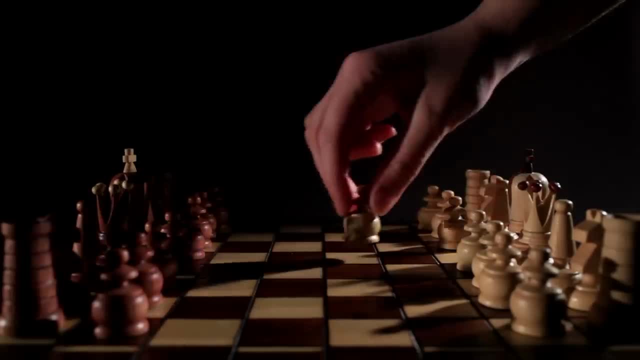 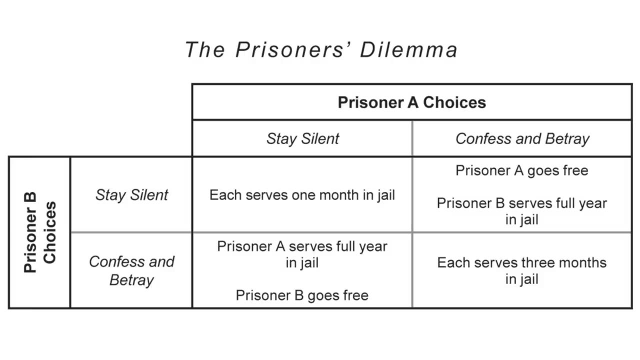 To summarize, it's about the study of logical decision making and strategy within competitive situations. One of the most famous quote games that came up in the early days of this field was the prisoner's dilemma, where you and a co-conspirator have been imprisoned for committing a crime. 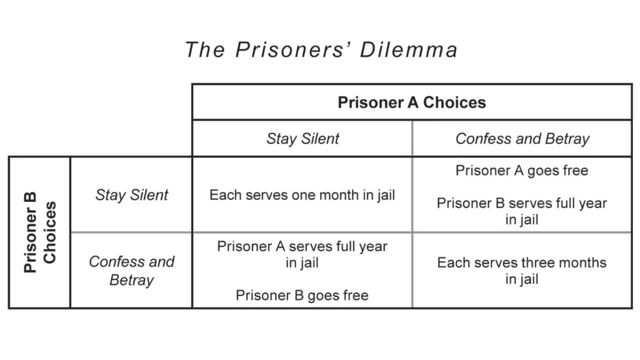 You're separated and each have the option to either stay silent or rat on the other and say they did it And, based on what each of you do, you may go to jail for a certain amount of time or you may be set free. 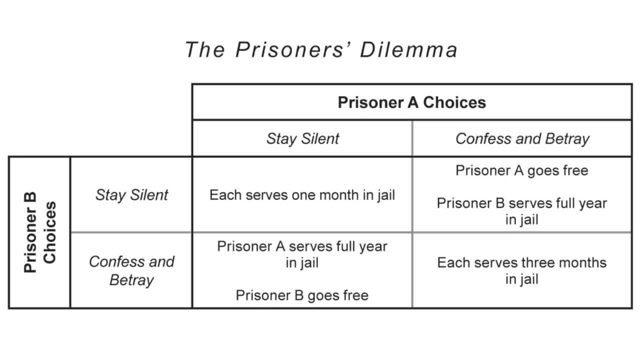 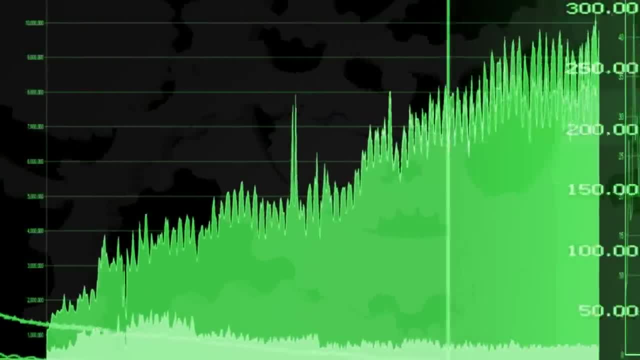 The question here is: what is in your best interest to do, especially while not knowing what the other person will say? This field grew to have applications in both economics and computer science, as well as a few other fields. In computer science, there's cloud computing. 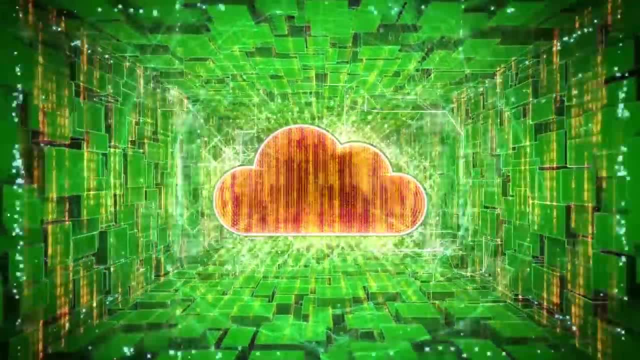 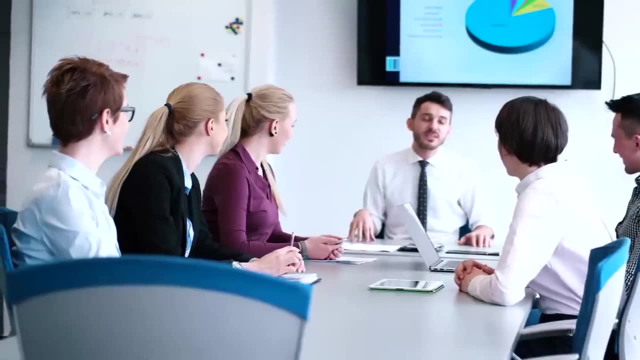 in which game theory can be used for modeling interactions between cloud providers, where costs should be minimized, while other factors maximized. In economics it applies to auctions, mergers and acquisitions, where each party wants the most benefit, financial analysis and a new product release. 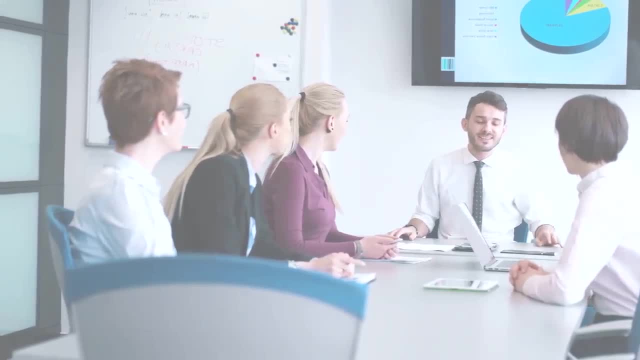 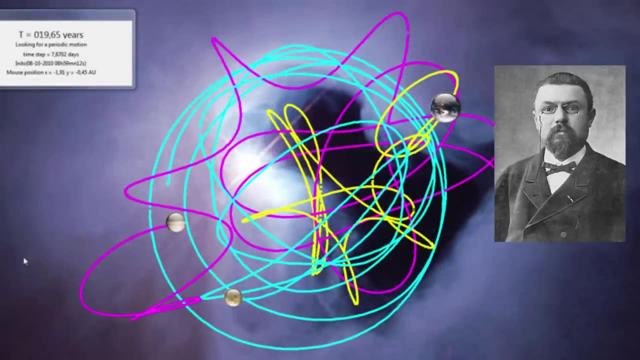 and much more. Then, in the 1880s, the mathematician Henri Poincaré was studying the three-body problem, which deals with studying the motion of three point masses, for example the motion of the Moon, Earth and Sun. 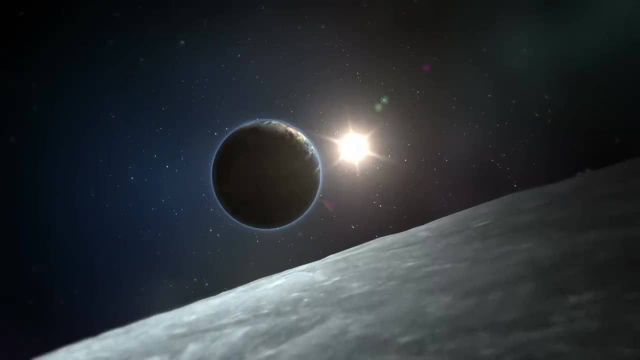 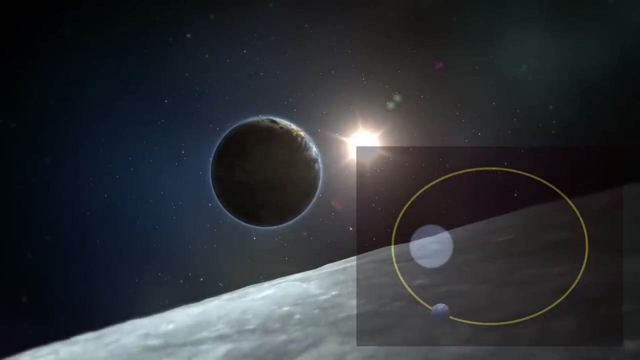 under each other's gravitational pull. Analyzing the motion of two orbiting bodies is very doable using Newton's laws of motion, but throw a third in and it actually gets very difficult. Now Poincaré found that small changes in the position. 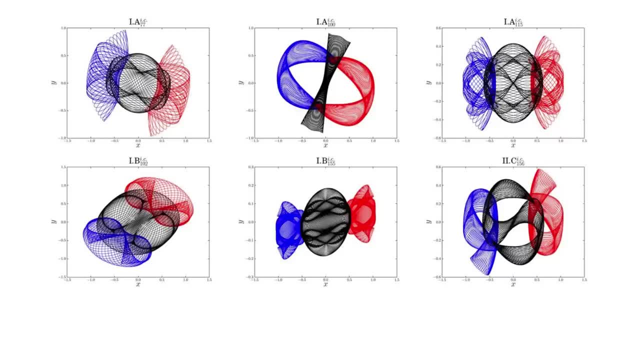 and initial velocity of these masses would cause for way different behaviors over time. This was the beginning of chaos theory, a field of math dealing with dynamic systems that are very sensitive to initial conditions. Now, after his contributions, the field slowed down a lot. 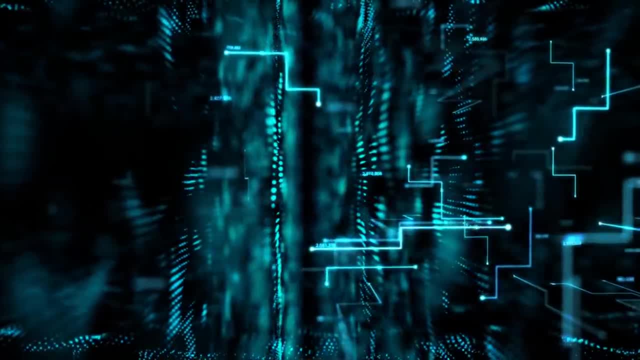 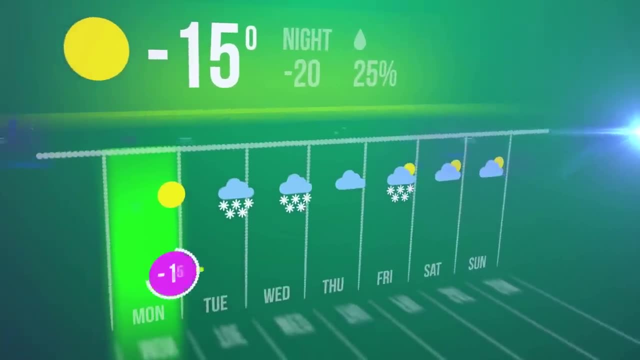 due to the lack of computational power back then. Eventually, a man named Edward Lorenz accidentally found his interest in this subject through his work in weather prediction in the early 60s. He realized that when he made a small change to initial conditions in a computer simulation, 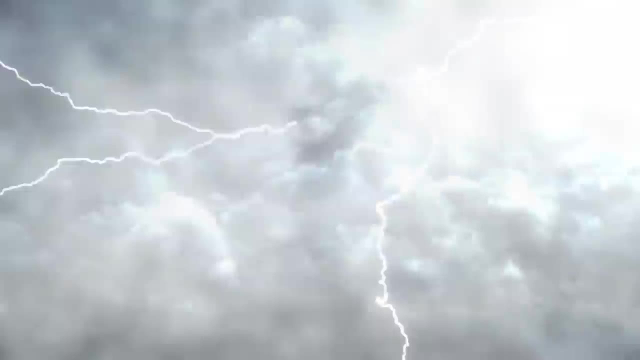 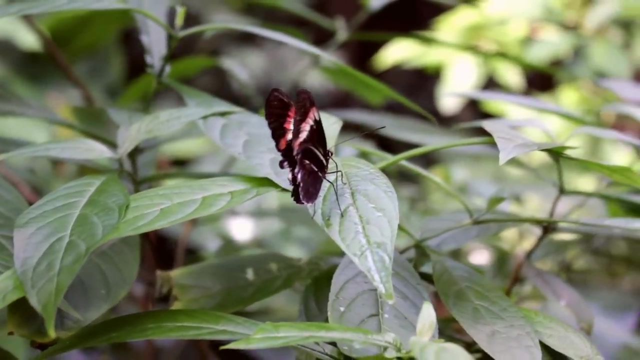 it produced huge changes in the long-term final outcome. You may have heard of the butterfly effect, a metaphorical example where if a butterfly flaps its wings on one side of the Atlantic Ocean, let's say, it could cause a tornado on the other side weeks later. 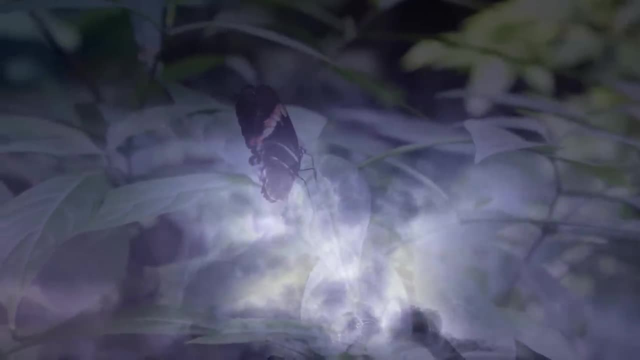 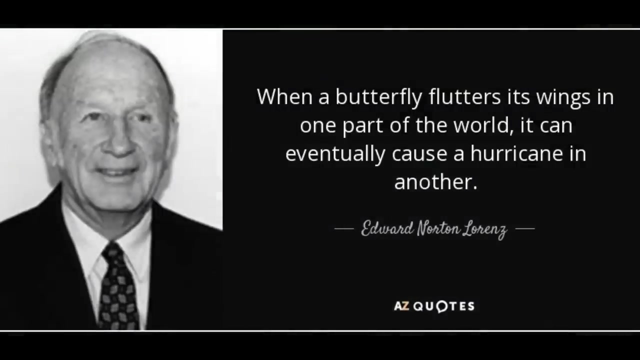 Well, this very minor change in the environmental conditions causing a large difference is a concept of chaos theory, and its name, the butterfly effect, was coined by that man, Edward Lorenz, after his findings with the weather simulation. The butterfly effect is a concept of chaos theory. 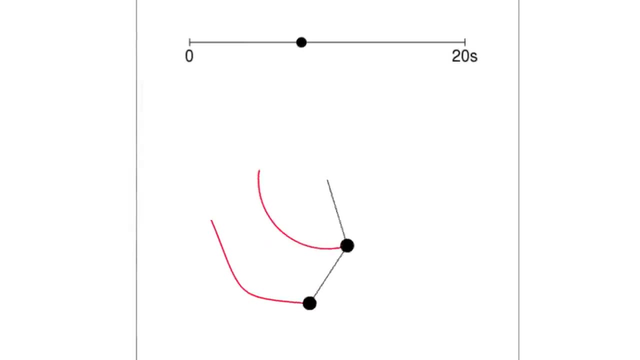 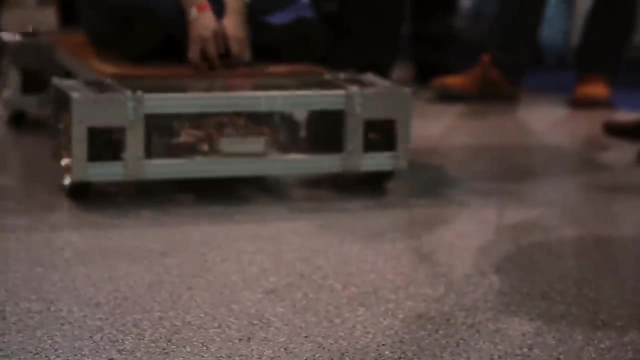 that is used to analyze systems like a double pendulum, where changing its starting height even a little greatly changes its path. It's used in robotics to predict the motion of a robot and how it will develop over time, and it can even be used in cryptography. 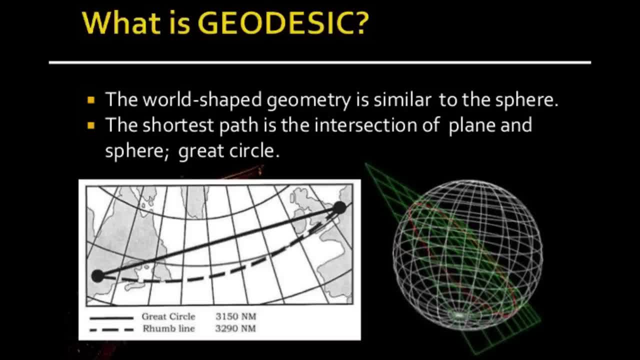 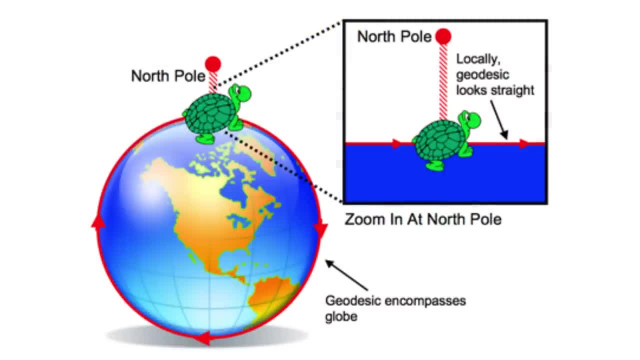 Next up geodesics are curves representing the shortest path between two points on a curved surface. These are what an ant living on the surface would perceive to be straight, and it explains why airplane routes on a map are curved a little. These are of huge importance for Einstein's general theory of relativity. 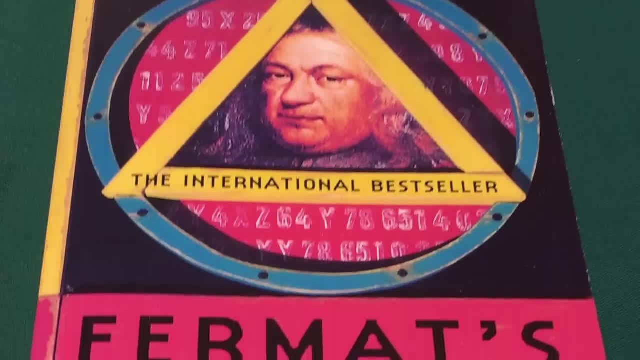 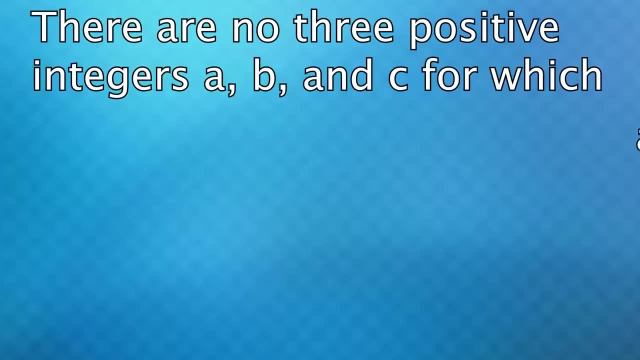 Moving on, Fermat's last theorem, which is easy to understand on the surface, was unsolved for 300 years. This theorem says that there are no three integers, a, b and c, such that this is true where n is any integer greater than 2.. 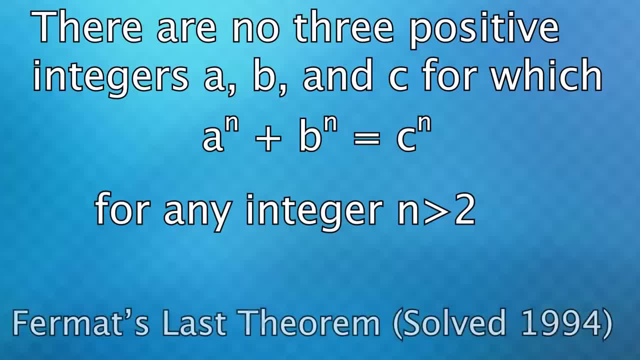 No one could prove whether this was true until just a few decades ago, in 1994, where Andrew Wiles finally proved the theorem and found that in fact there are no integers that make this true, And although the theorem is easy to understand,